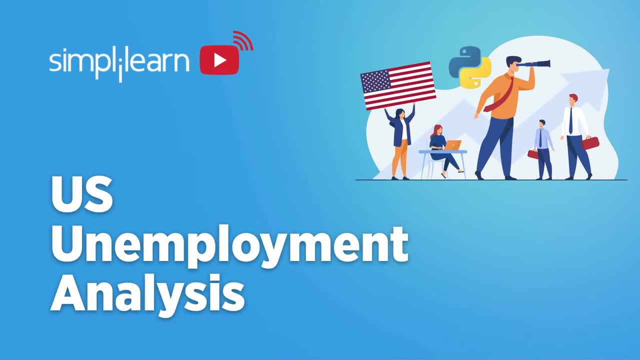 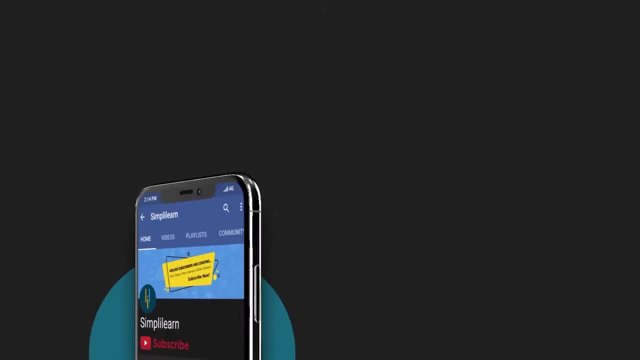 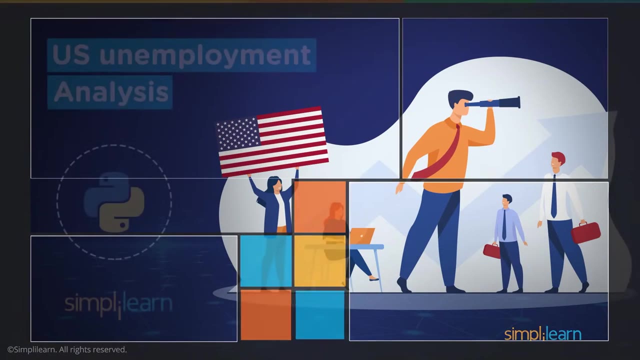 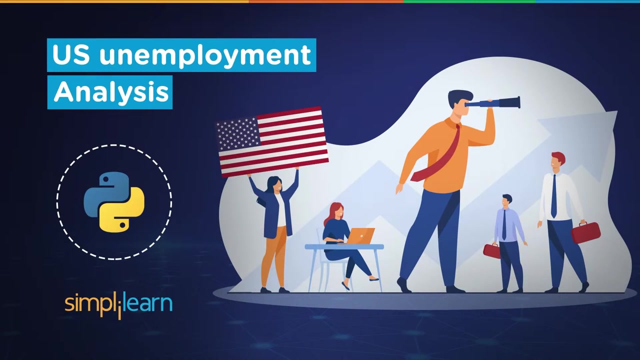 Hello everyone and welcome to yet another interesting live session on the series of sessions related to data analysis in Python. In this video, we will be analyzing and visualizing the United States unemployment dataset from 1948 to 2021.. This data has been collected. 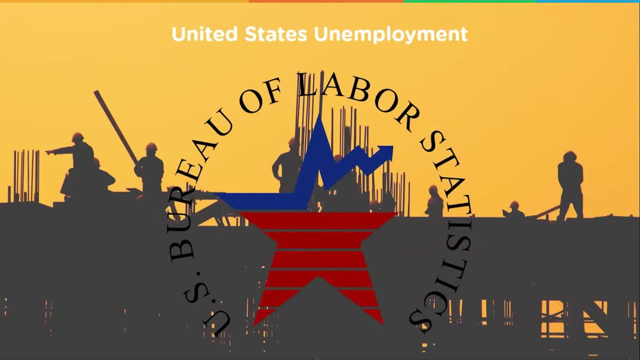 from the United States Bureau of Labor Statistics. The data contains the monthly unemployment rate from 1948 to 2021.. The file also contains information on subsets of the population that includes based on age ranges from 16 years of age to 55 years of age and above, And it 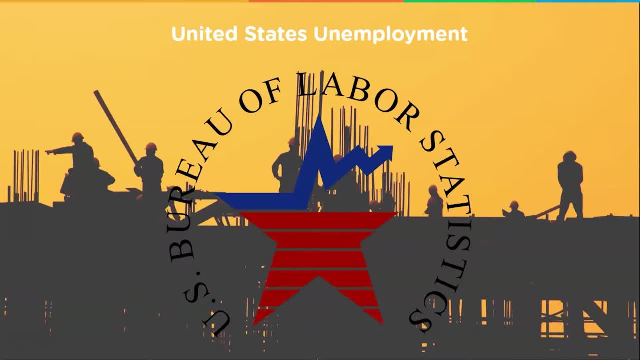 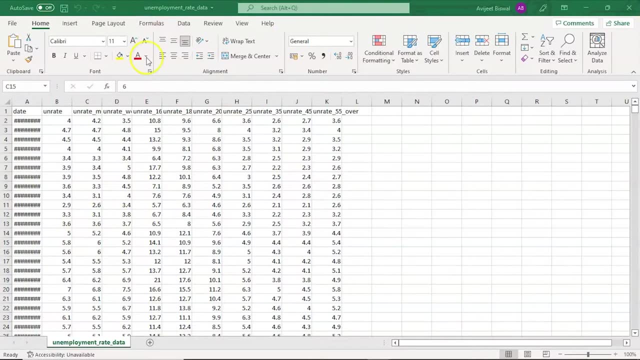 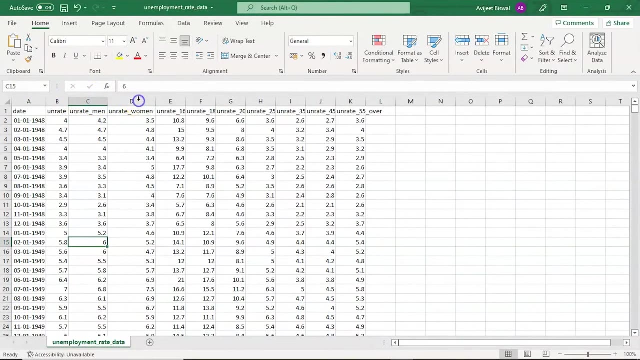 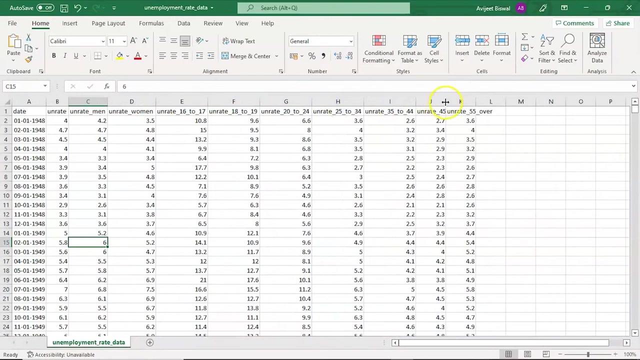 also has information about unemployment rates for men as well as women. Now let me go ahead and show you the dataset first. On the screens you can see the unemployment rate data. Let me just adjust the column headers so you know the different columns that we have, If you 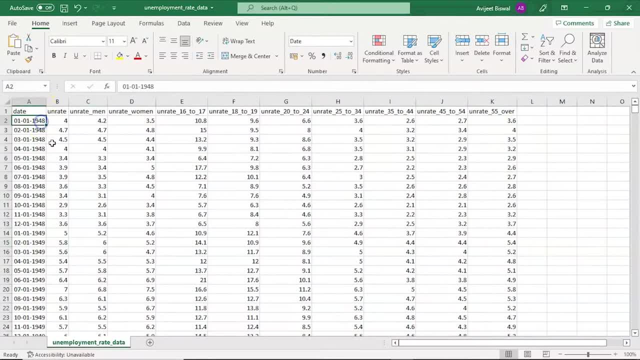 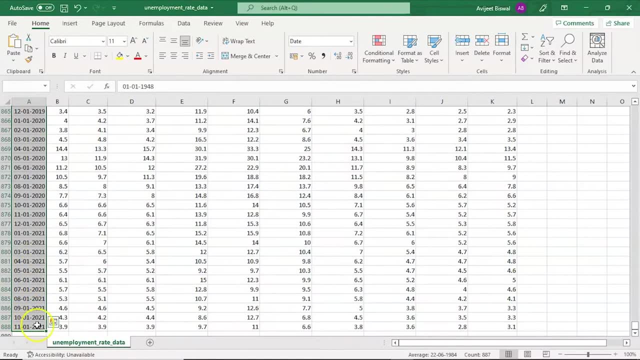 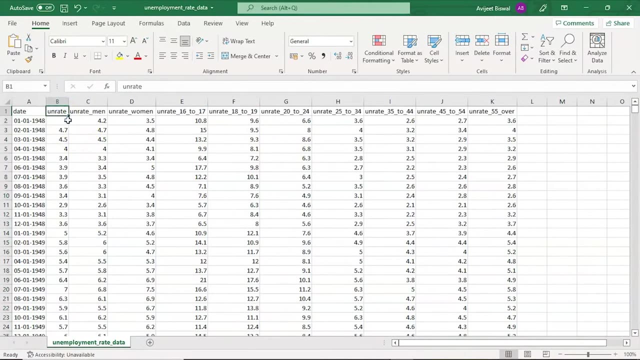 see, the first column is of date, so it starts from 1st of January 1948 till we have data till November 2021.. Okay, go to the top. Then we have the overall unemployment rate. The next column we have is the overall unemployment rate for men over these years. Then we have 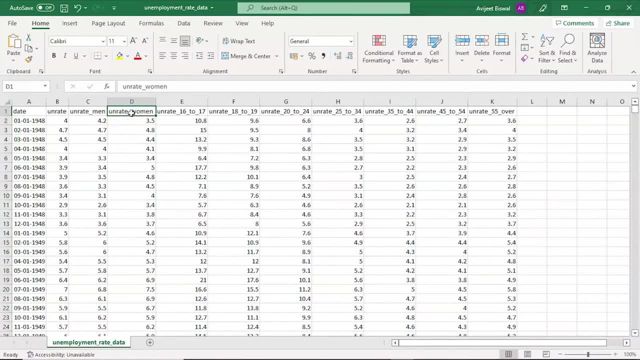 the overall unemployment rate for each of the months starting from 1948 to 2021 for women. Next, we have the different age groups. so unemployment rate For the younger people, 16 to 17 years of age, then we have between 18 to 19, then 20. 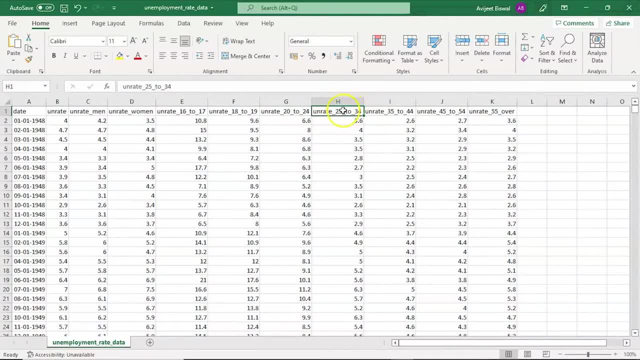 to 24,, 24 to 34.. This is actually 25 to 34, then 35 to 44,, 45 to 54. Then the last column is 55 and above. Alright, so we are going to use this dataset and we'll be analyzing. 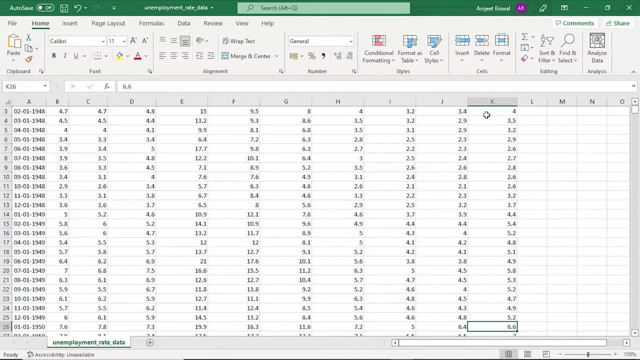 for three specific periods between 1980 to 1990.. We'll focus on the Great Recession of 2010 and we'll also be analyzing the post-COVID data. So, to give you a context, the early 1980s recession was an economic recession. that affected much of the world between the start of 1980 and early 1983. So it was one of the severe recessions since World War II. A key reason for the recession was the 1979 energy crisis, mostly caused by the Iranian revolution, which caused a disruption in the 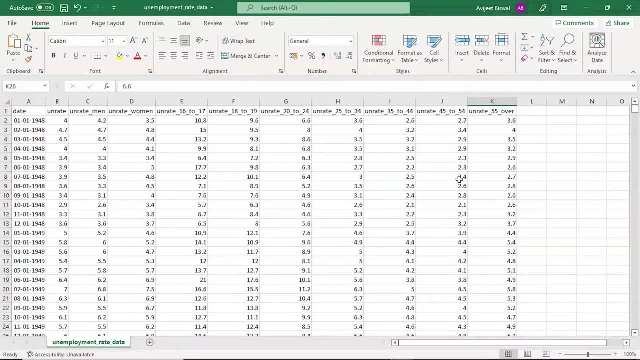 global oil supply, So that saw the oil crisis rising sharply in 1979 and early 1980.. Then we'll focus on the second period, which is the Great Economic Recession. that refers to the economic downturn from 2007 to 2009 after the bursting of the United States housing. 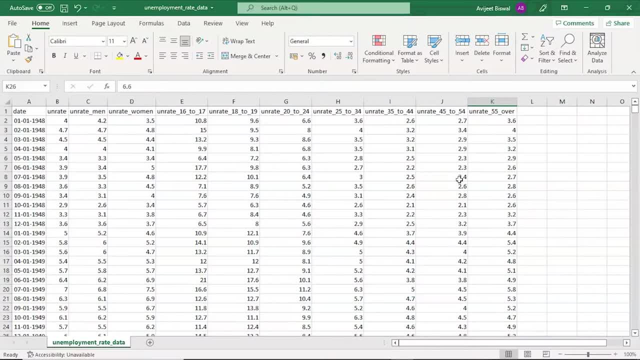 bubble and the global financial crisis. The Great Economic Recession was the most severe economic recession in the United States since the Great Depression of the 1930s. And finally, we'll focus on and analyze data of 2020, when the world was hit by the global coronavirus pandemic. So the pandemic did. 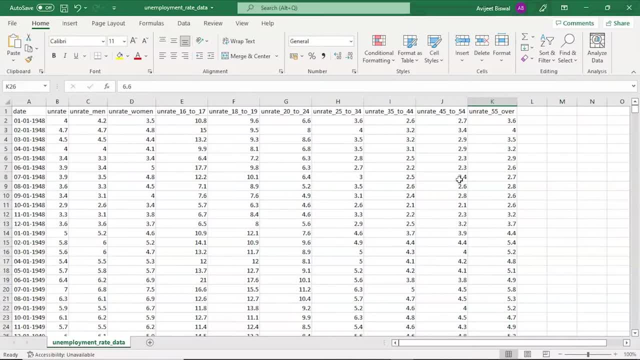 not only impact the human lives, but it also shook the economy and job market of infected countries. So let's head over to our Jupyter Notebook and we'll start with our demo session with importing this dataset. So for that, let's go to our Jupyter Notebook and we'll start with our demo session with. 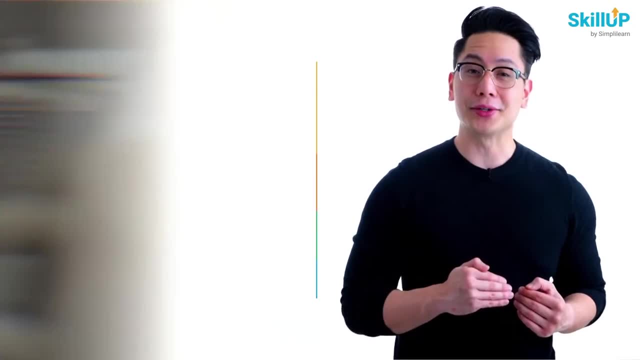 importing this dataset. So for that, let's go to our Jupyter Notebook and we'll start with importing this dataset. So for that, let's go to our Jupyter Notebook and we'll start with importing this dataset. So for that, let's go to our Jupyter Notebook and we'll start with importing this dataset. And that means we'll already have the dataset. theğan sen ships that are grabbed last 30 million years ago have made젠as following theodles from India. If getting your learning started is half the battle, what if you could do that for free? 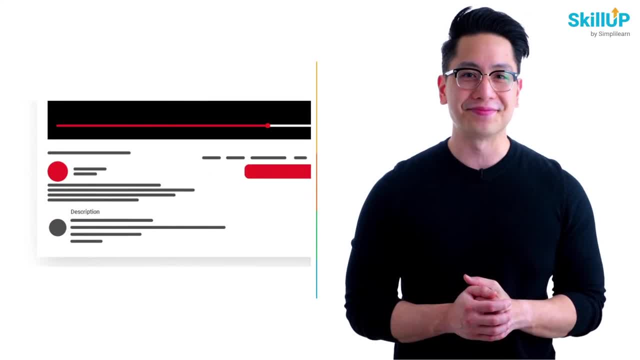 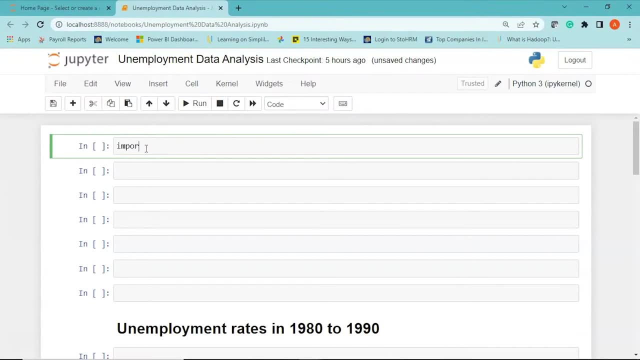 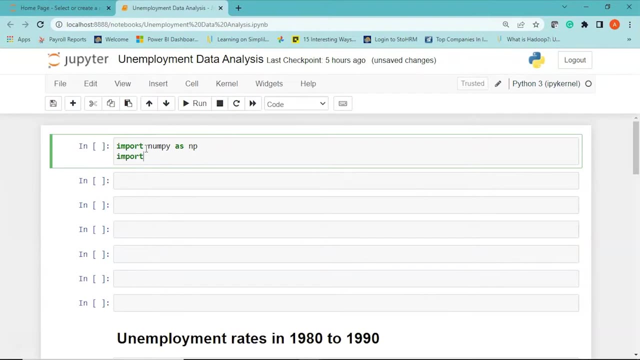 Visit SkillUp by SimplyLearn. Click on the link in the description to know more. I'm going to import the necessary libraries first, So I'll start with import numpy or numpy as NP, And then I'll have import pandas as pd, And then I'll import a lot of options for it. 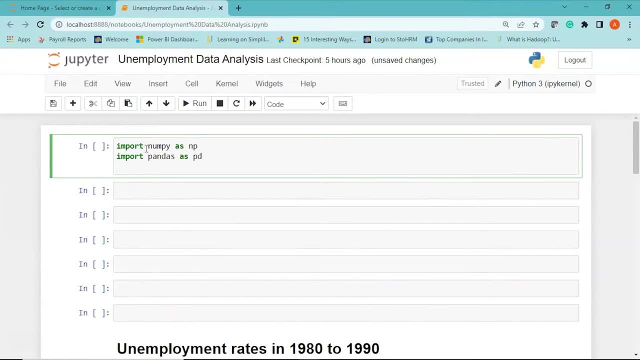 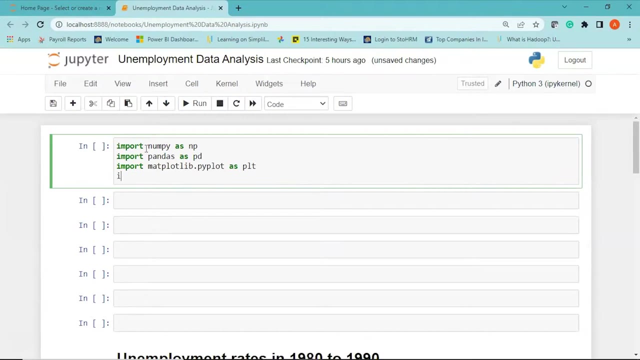 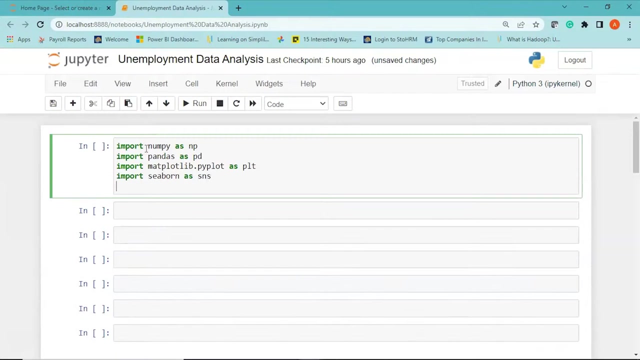 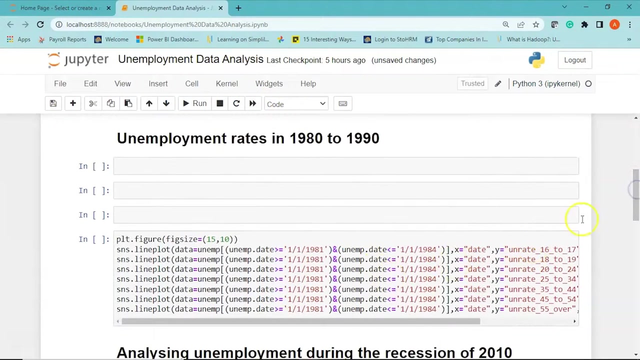 Humph. So first of all I have to have the code for istiyorum ethos formula and then i'll import matplotlibpyplot as plt. next i am going to import seaborn as sns, followed by, i'll say, percentage matplotlib inline. okay, so this is the notebook that i'm going to use. if i scroll down, you would see some of the cells. 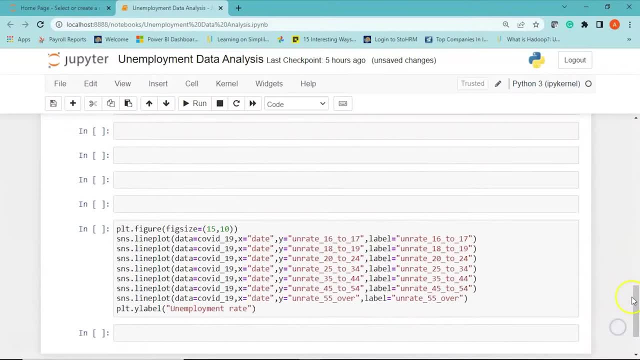 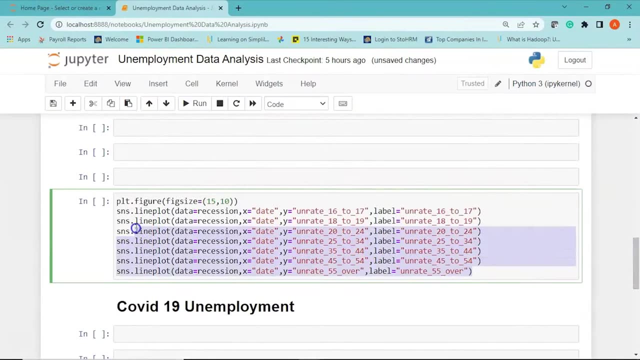 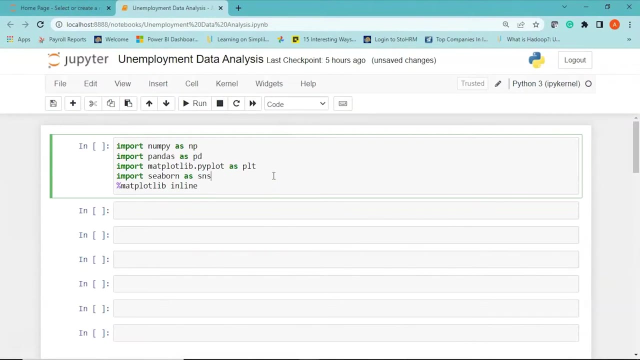 already filled. i will come to this later. i just wanted to make sure that we have enough time to explore this data set and try saving some time writing the same lines of code again and again. okay, so let's go ahead and import all the necessary libraries. i'll hit shift enter. 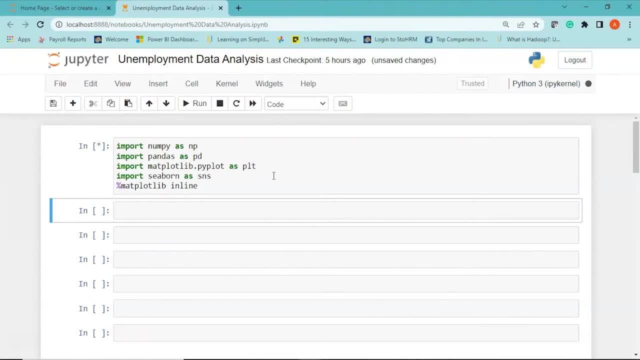 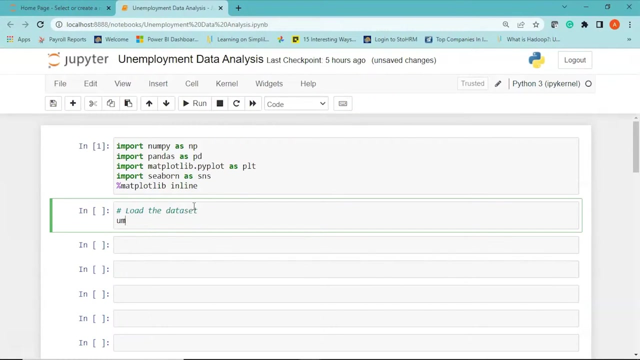 now you can see we have successfully imported all the necessary libraries. the next step is to load the data set, so i'll give a comment. load the data set. so i'll store my data set by converting it into a data frame with a variable called unemp, which basically stands for unemployed. so i'll use the function read underscore: csv. 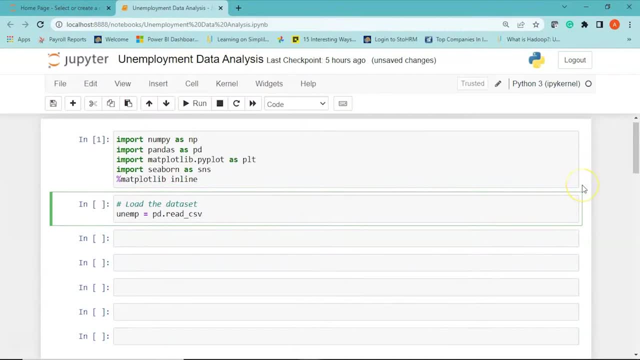 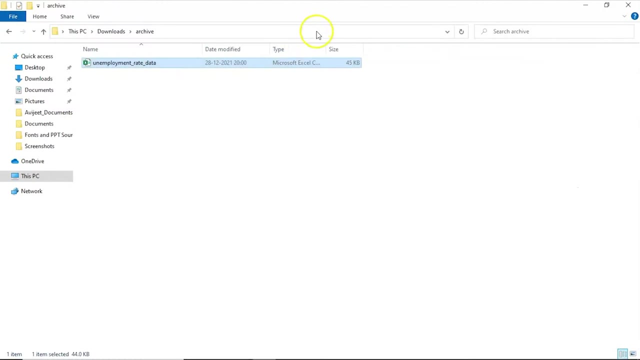 because the data set that we have, or that we looked at, was a csv data set. after that, within quotations, i need to pass in the file location. so let me just go ahead and copy the file location. just click on this and here we'll copy the file location and we'll see that we have. 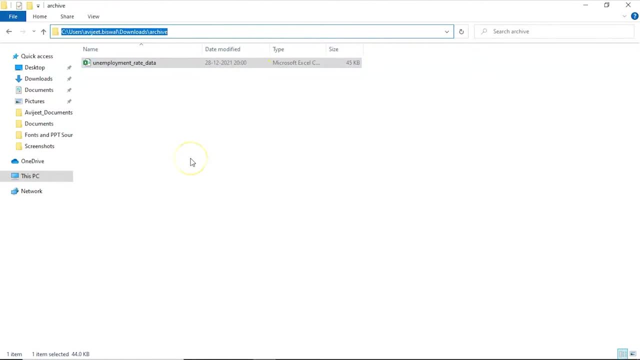 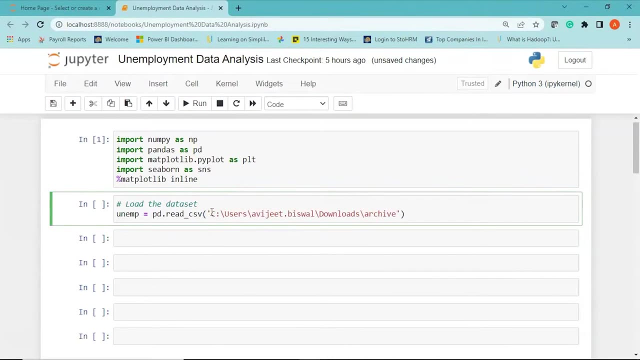 copied this file location and i'll paste it. i'll click here and i'll paste the location that we just copied. make sure we have another backslash, otherwise it won't read on a windows system. i'm using a windows system here, all right. after that, i'm going to give the file name, along with the extension of the file, that is. 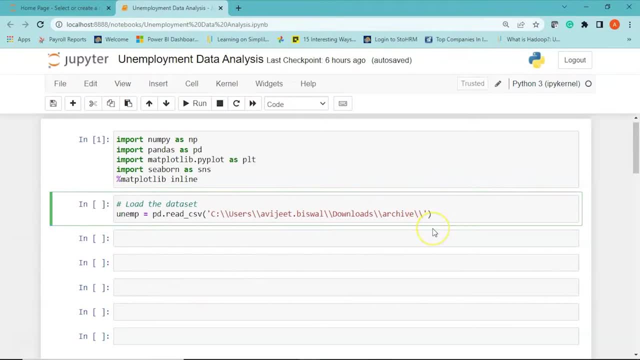 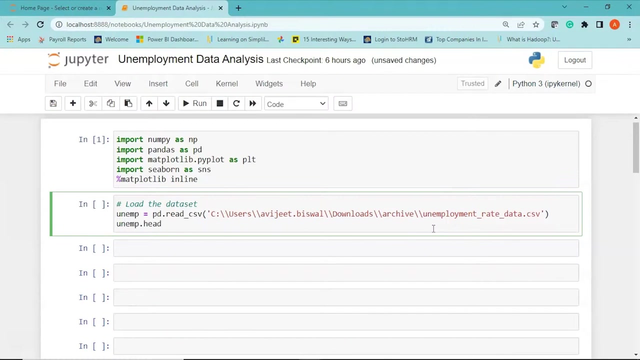 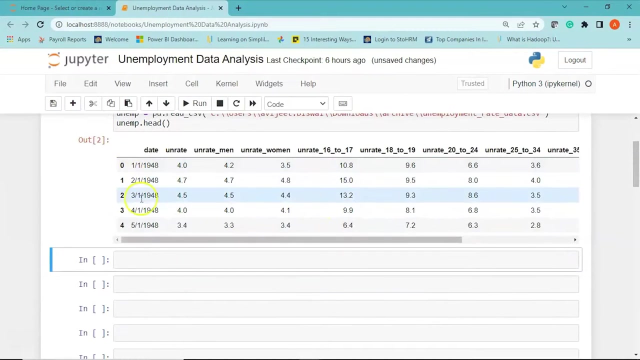 csv. here i'm going to give the file name, which is unemployment, underscore, rate, underscore data dot csv. actually, data dot csv. okay, this looks fine. and to print the first five rows of the data frame, let me just use the head function, so i'll say unemployment dot head. let's run it okay. so here you can see the output below. so we have the first. 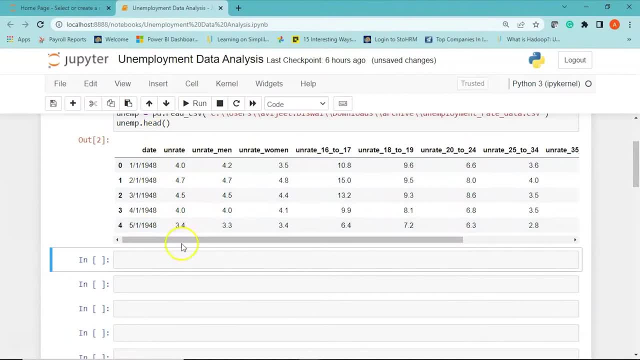 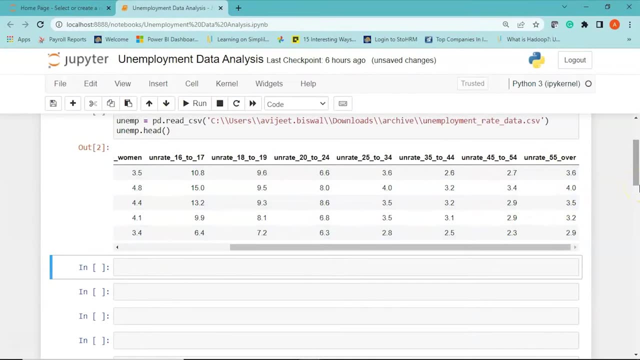 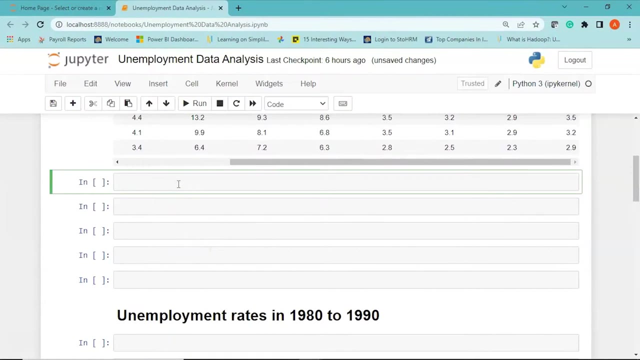 five rows from the data frame. it has all the columns starting from the date column till the last column, which is unemployment rate for 55 years and above great. now, in the next cell, let's check the data types of each of the columns that we saw and the non-null values. 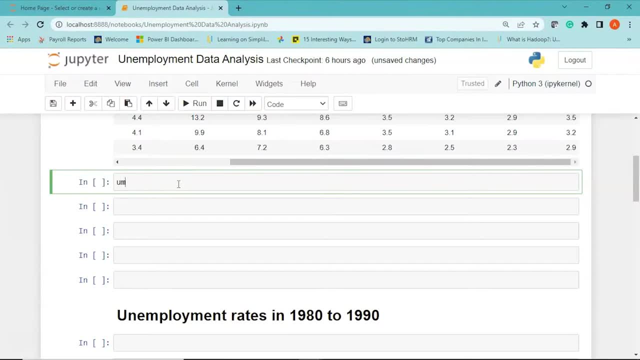 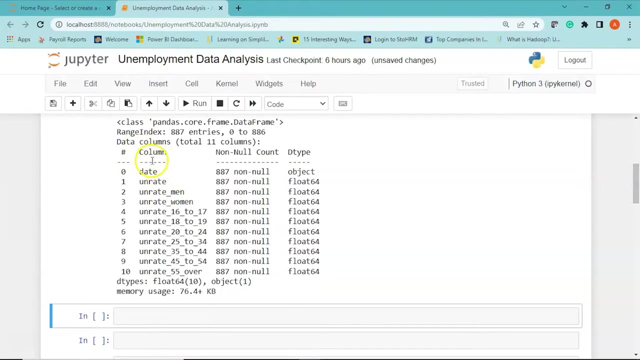 as well as the memory usages. so for that i'm going to say unemployment dot info. right shift enter. you can see here i have different column names. on the top you can see there are total 887 entries as in. there are total 887 rows in my data frame, starting from 0. 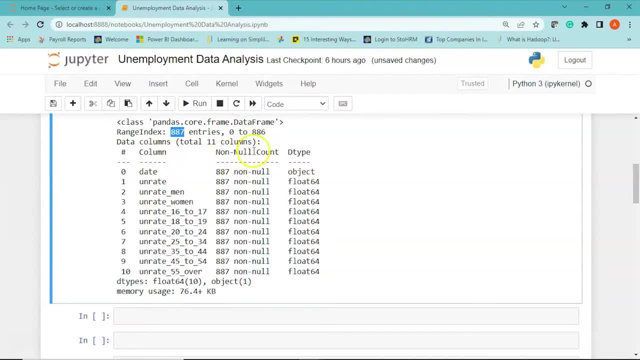 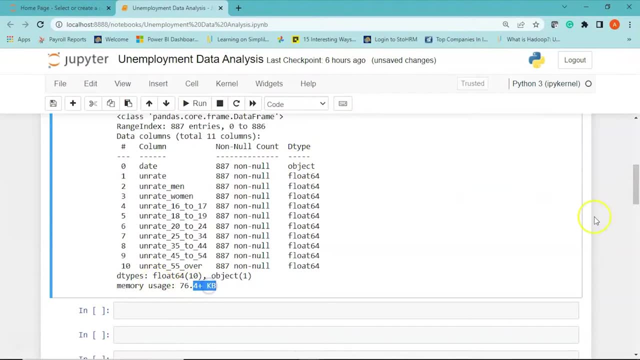 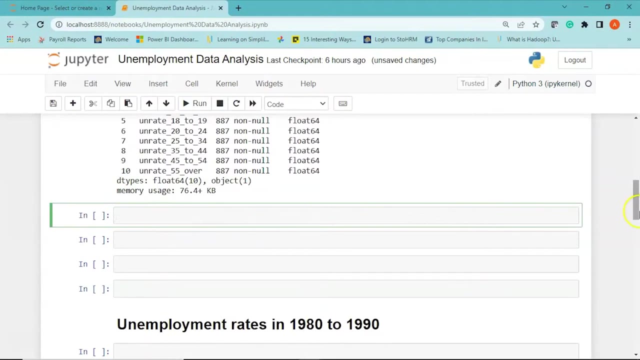 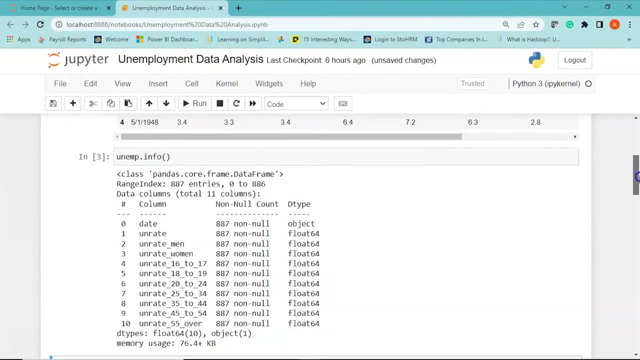 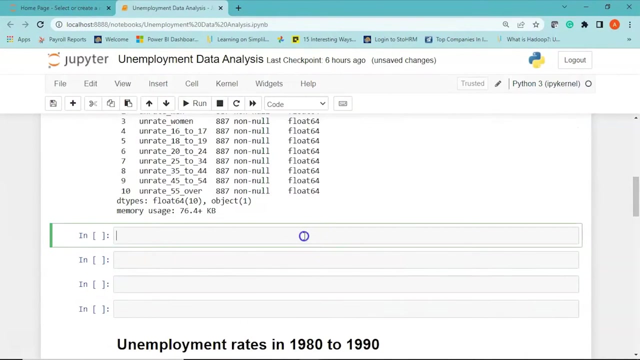 to 886. we have the different columns, the non-null count and you have the data type here and at the bottom you can see the memory it is using- cool. next we need to convert the date column- that is the first column- into date format or date time format. for that we need to make some changes. so i'll say: 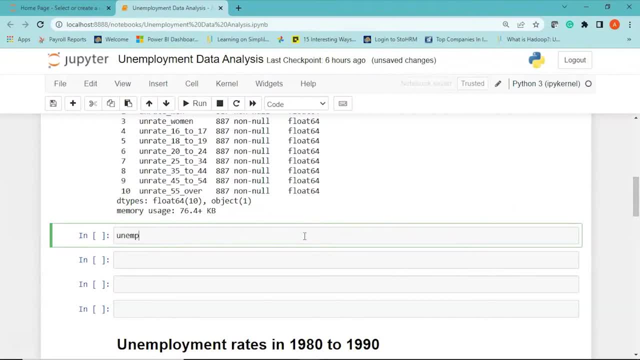 unemployment, which is my data frame name. within brackets i'll see my column name. that is date equal to pd dot to underscore date time, which is the function, and i'll say unemployment and i'll pass in my column that is indeed. next, let's use the describe function. i'll say unemployment. 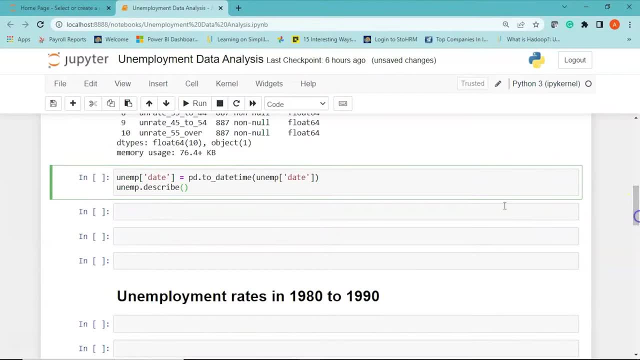 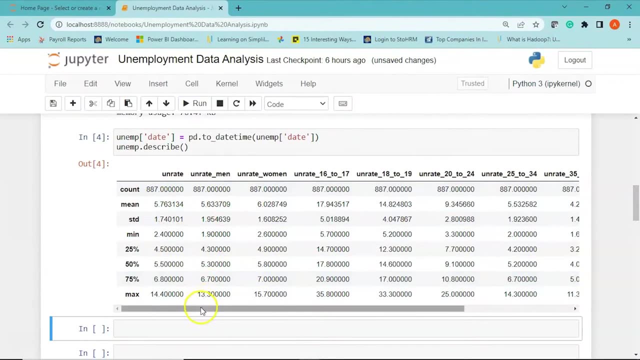 dot describe, to get some statistics which will get us some statistical outputs. there you go. so here you can see the count for each of the columns, that is 887, and then for each of the columns we have the minimum value, which means the overall unemployment rate starting from 1948 to 2021 in the united 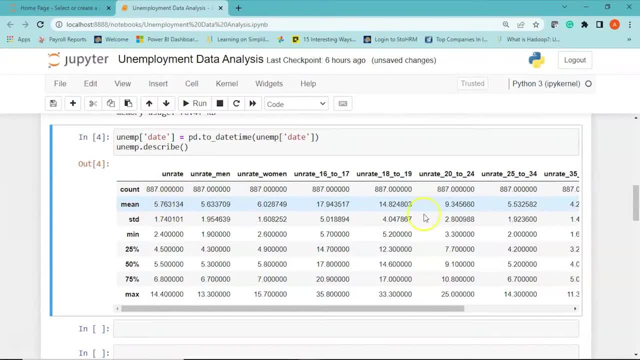 states has been around 5.7 percent. and then if you check the data here, you can see that check for the unemployment rate for men, the maximum it has touched is 13.3%- I believe this is during the COVID pandemic- and the lowest is 1.9%. Again, if you check for women, the highest 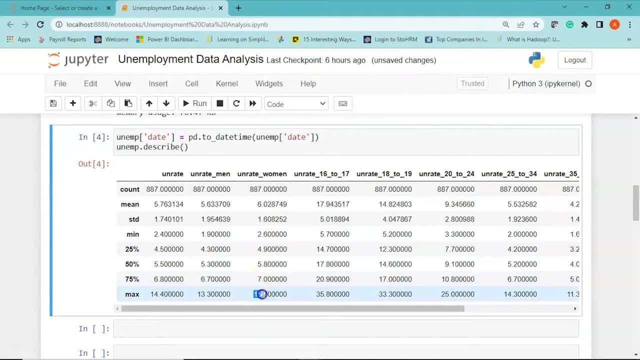 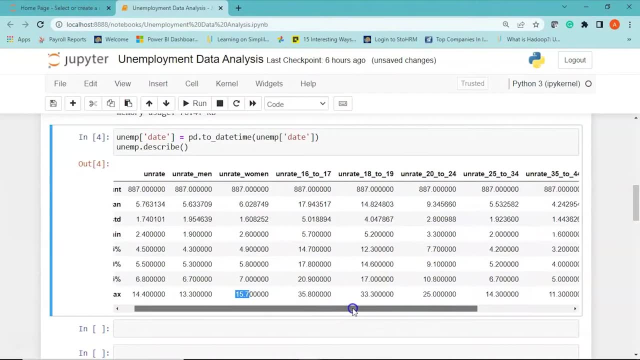 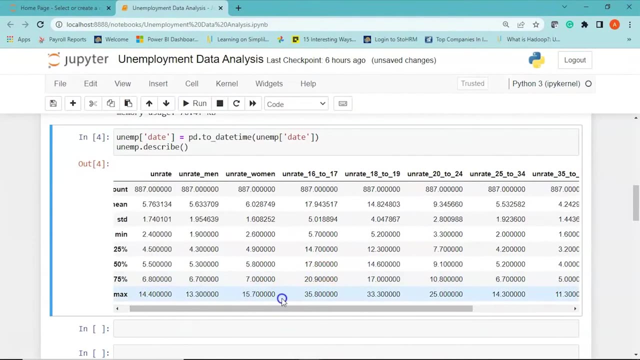 unemployment rate in women has touched 15.7%, which is again during the COVID pandemic. And then we have the unemployment rate for the age groups. Now, if you see the maximum value for the different age groups, you find that there are more unemployed people between 16 to 17 years of. 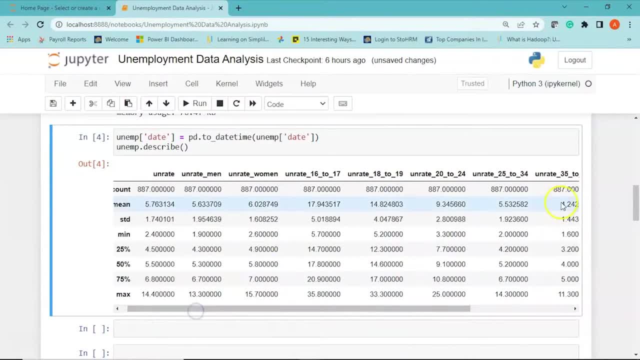 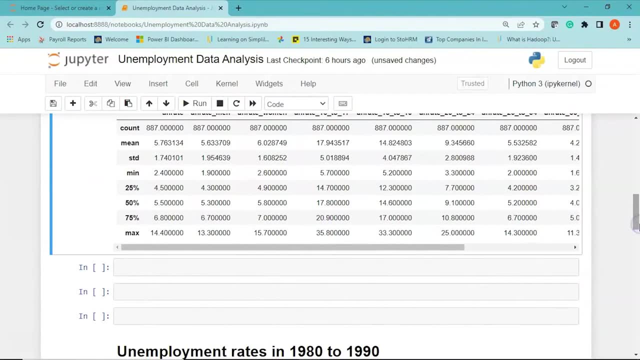 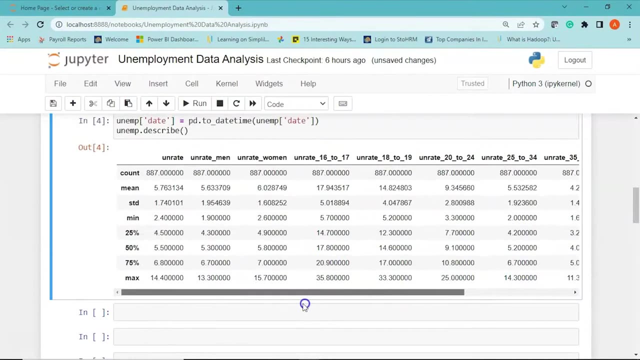 age, that is, the younger population, are the ones who are mostly hit by the unemployment in the United States. Okay, Now moving ahead With that. I just wanted to call it out again that, historically, what we see is that 6% of women 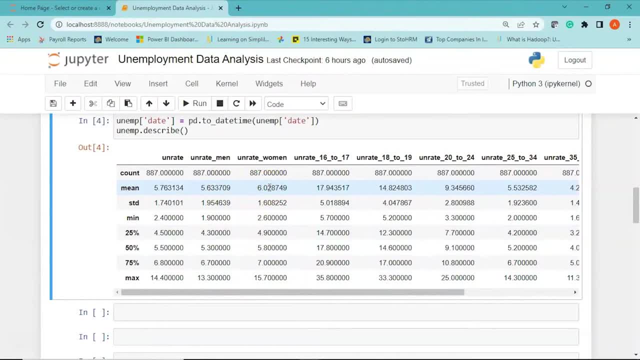 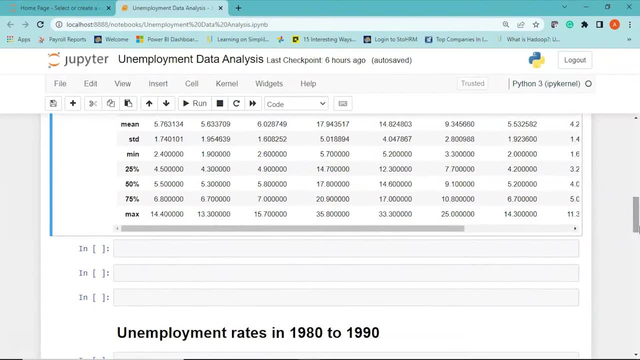 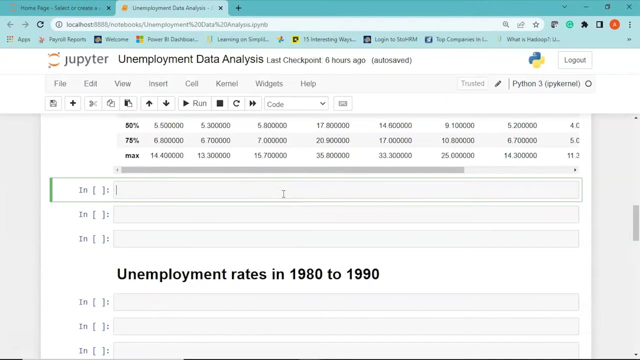 on an average have been unemployed as compared to 5.6% of men. Let's visualize the overall unemployment rate. So here we are going to create our first visualization now and that would be a line chart. So I'll say PLT dot figure. 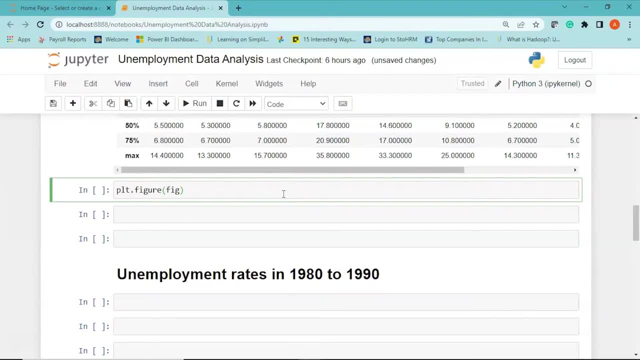 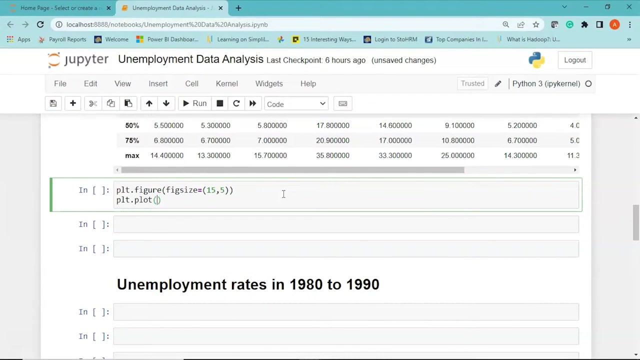 then square brackets, I'll write figure size. Let's say we'll give the figure size as 15,5.. Okay, Next I'm going to say PLT dot plot to plot my line chart or line graph. then I'll pass in my data frame that is unemployment. 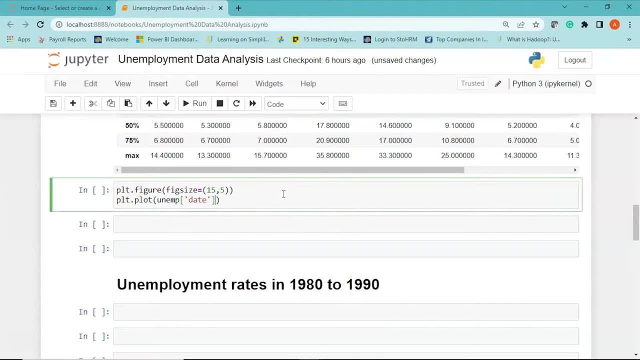 I'll call my date and then we'll have employment rate column. So again, I'll pass in my data frame name. within square brackets I'll say unrate. If you see the first column here, this is the unemployment rate. 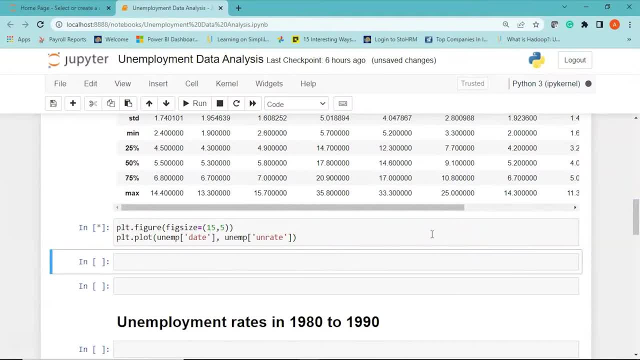 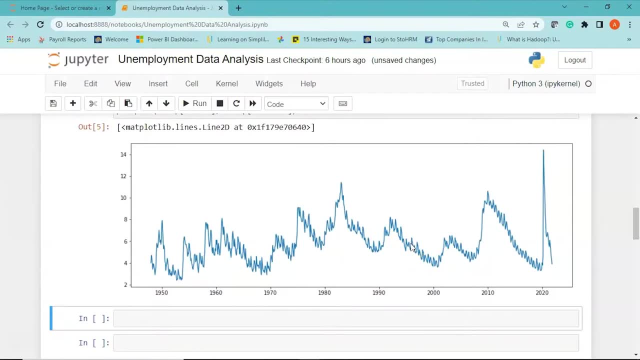 that is the overall unemployment rate. Let's go ahead and run this. It will plot this line chart For us. now what you see is there are three instances of high unemployment in the United States. One is between 1980 to 1985.. You can see there's a clear spike, And then 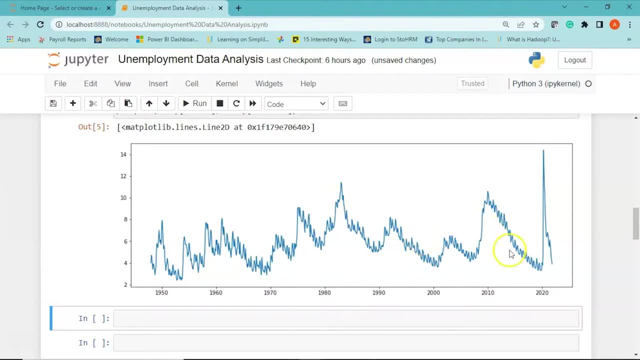 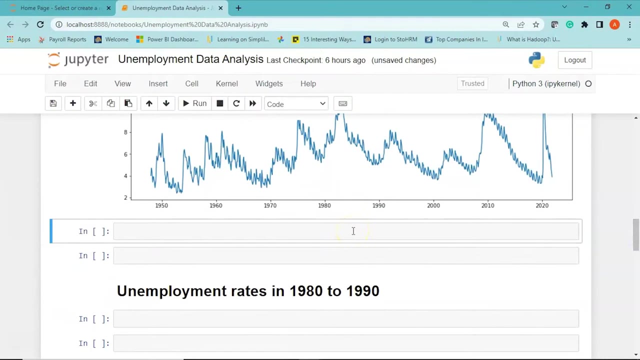 the second instance is between 2010 to 2015.. There's again a clear spike, and the maximum spike in the unemployment in the United States is after 2020.. That is the time when the world was hit by COVID pandemic. Cool, So we'll be focusing on these regions, or? 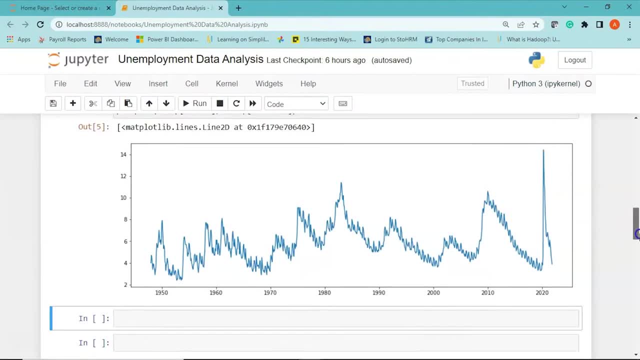 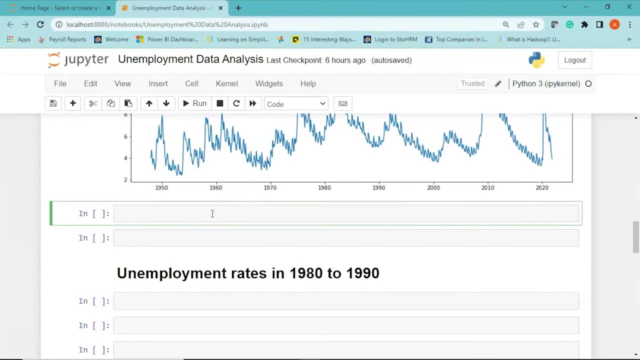 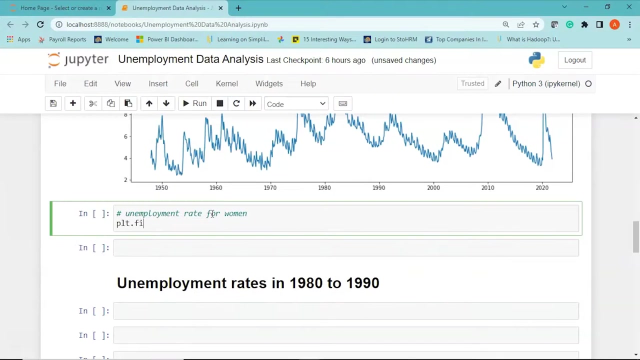 these time periods specifically in our analysis. Now, next we want to find the unemployment rate for women. So I'll just give a comment: unemployment rate for women, That I'll again say pltfigure. within brackets I'll say figure size to be. 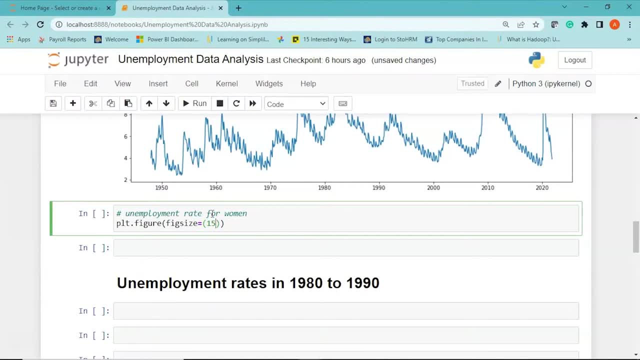 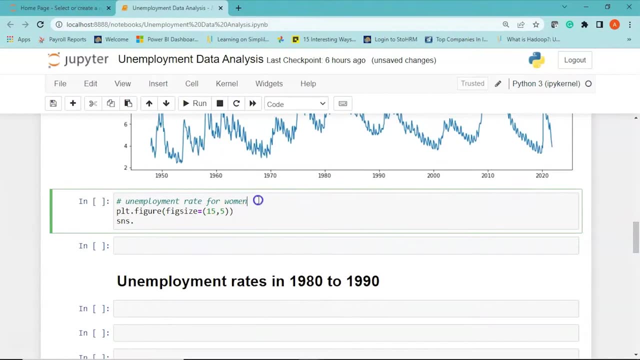 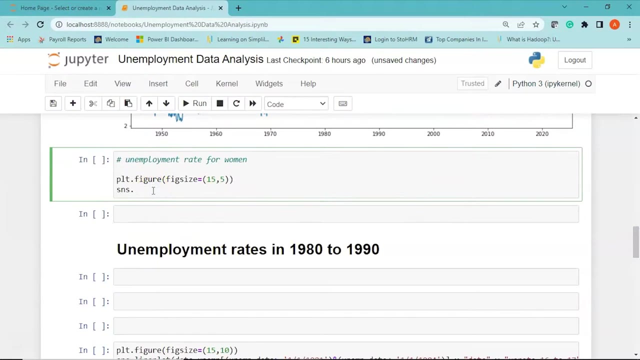 equal to 15,5.. And then I'm going to use the seaborn library and the sns abbreviation. So I'll say sns. I'll say line plot to plot the unemployment rate With my line graph. within brackets I'll say data equal to my data frame name that. 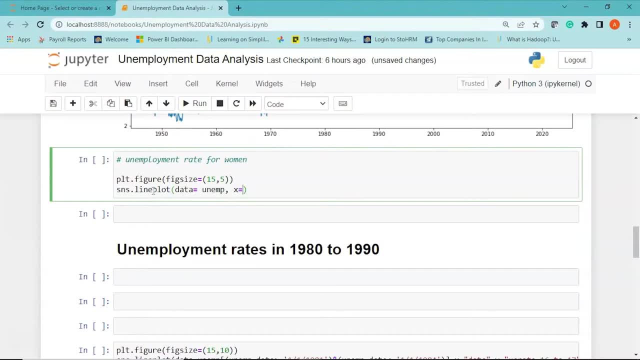 is unemployment comma In the x-axis. I want the date column In the y-axis. I want the unrate underscore women column to give me the unemployment rate for women starting from 1948 to 2015.. Let me write that to be 2010,, 2021.. And then you can also use a color. Let's say: use color. 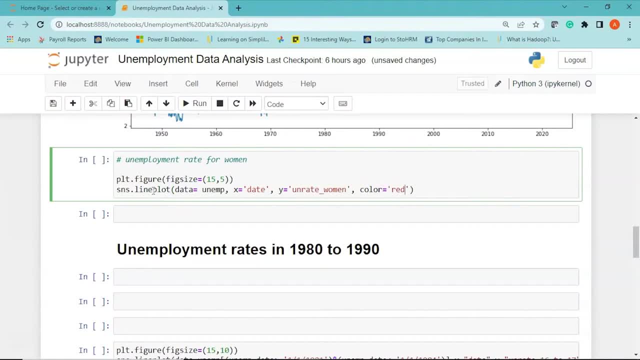 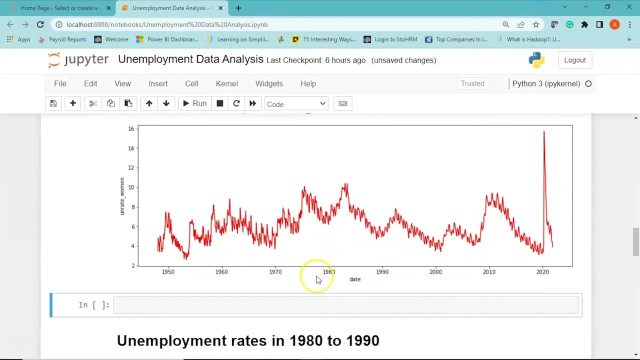 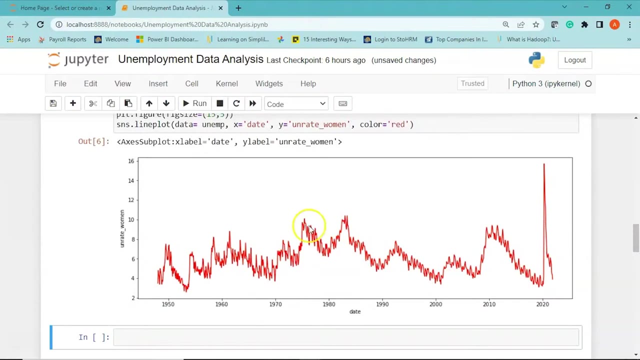 equal to red. Now we'll run this And let's see the output. Cool, You can see here the total unemployment rate of women starting from 1948 to 2021.. And again you can see there are clear spikes around these regions, whereas the world's unemployment rate is similar. And then, as I complete my analysis, I can see that the total unemployment rate of women in 2021 is about 1.2%. So the total unemployment rate is about 1.2% And I will divide it into the terms of the third place here. We can add a quote here: the third place here. So let's. 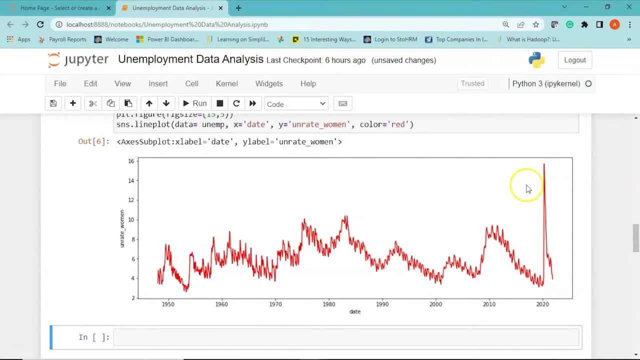 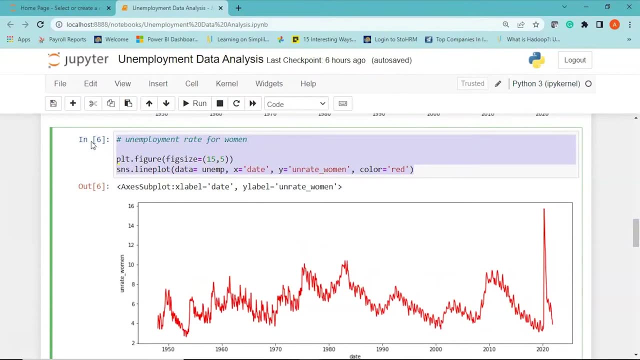 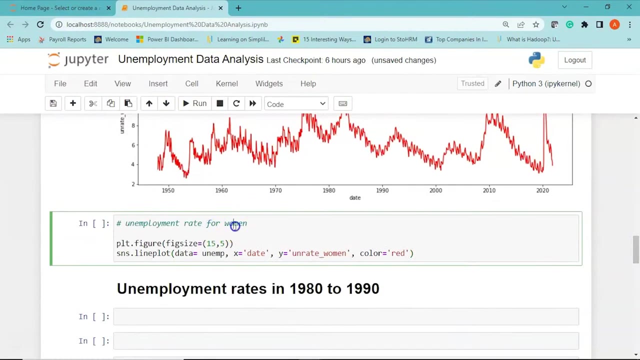 world. even the United States economy was hit by a crisis. Similarly, let me just copy this and we'll now check the unemployment rate for men. That is the overall unemployment rate. I'll just edit this: Data remains the same. My X axis remains the same. In the Y, 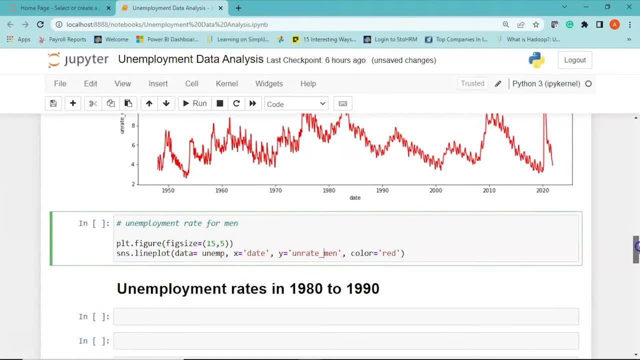 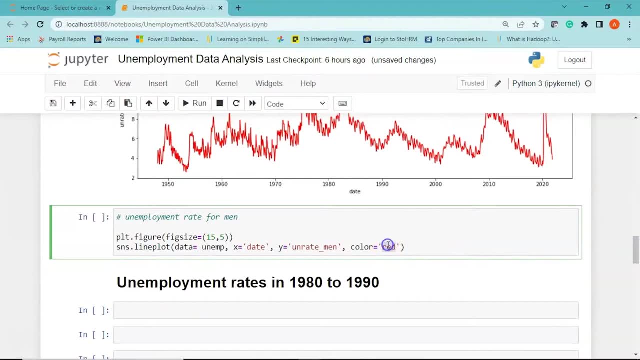 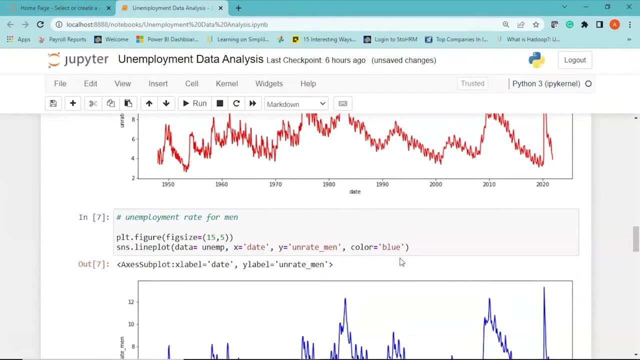 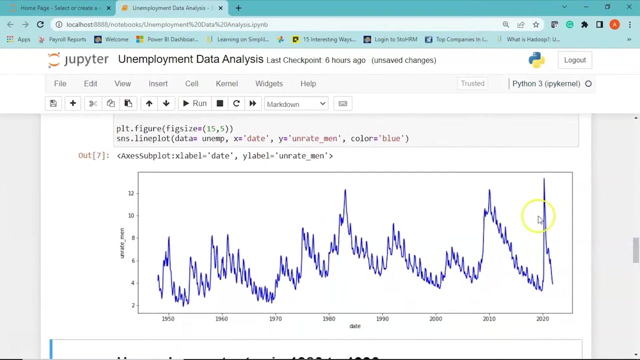 axis. I'll say unrate, underscore men. That is this column, Okay, And maybe we can change the color to, let's say, blue. Now let us run it, And here you can see for men: during the COVID pandemic, the unemployment rate for men reached almost. 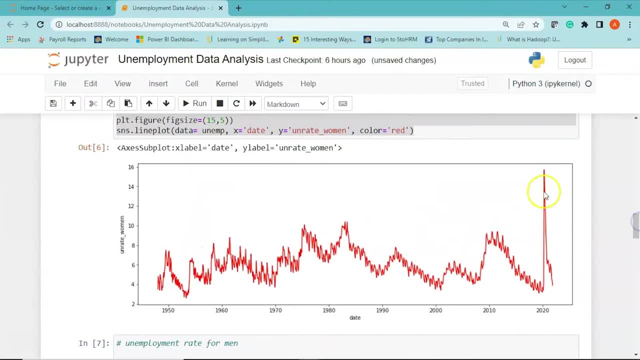 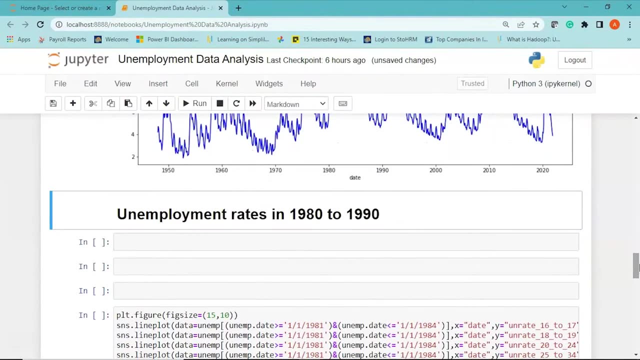 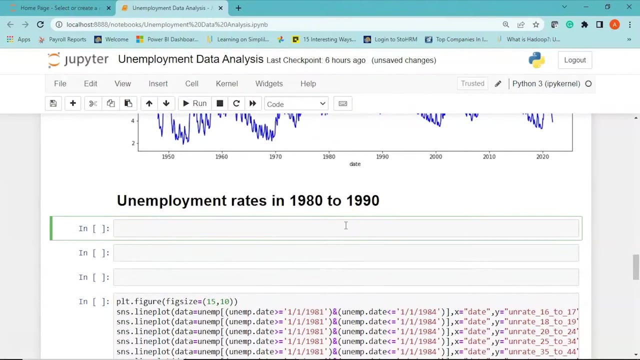 1%, Over 13%, And if you check for women, it was highest, which is close to 15 and above. Cool, Now we come to our first unemployment category. that is, between the 1980 and 1990.. So let's start with our line chart. So I'll first give the figure size, I'll say: 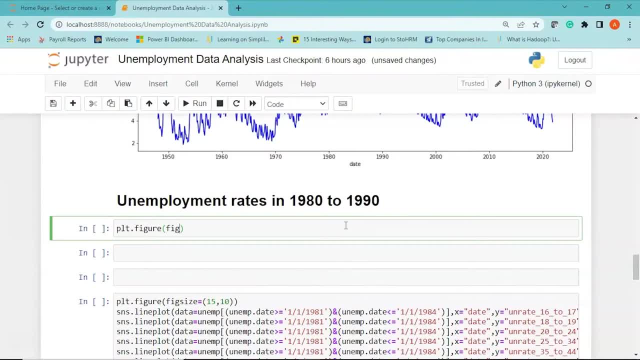 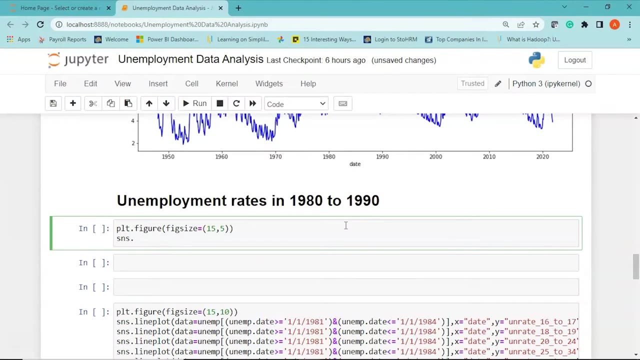 PLT dot figure Within square brackets. I'll say fig size That is equal to, I'll give 15 comma 5.. Now I'll say SNS, easily pig edged to 100 on the bright side and the data edge. 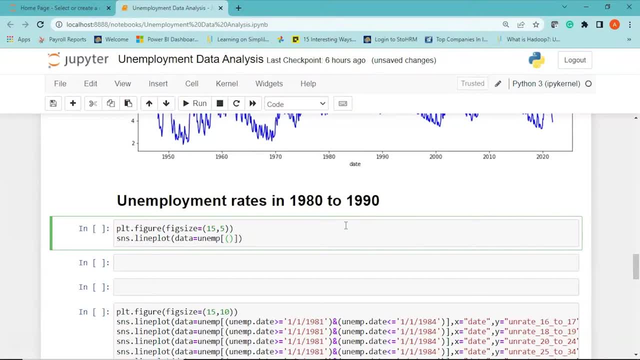 Isn't that nice. There we go. That's a nice look, our data frame, the original data frame. so for that I am going to say data equal to unemployment, and within square brackets I will give parenthesis. I will again say unemployment, dot date should be greater than equal to. I will pass in my date to be, let's say, 1st of Jan 1980, and then 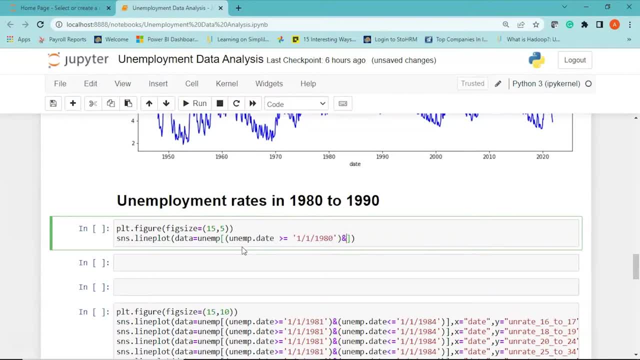 I will say ampersand, I will start another bracket. I will say unemployment dot date should be less than equal to, let's say, 1st of December 1984. so this is the time period that we are looking at, starting from 1st of Jan 1984.. 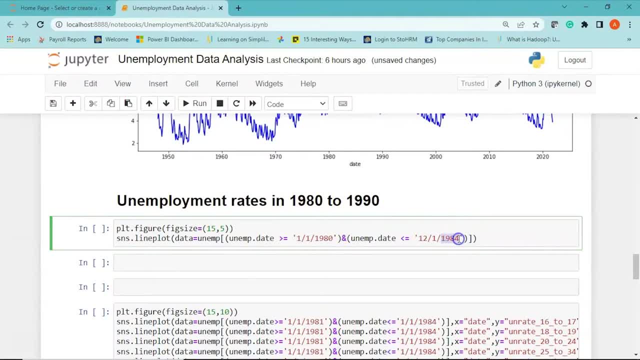 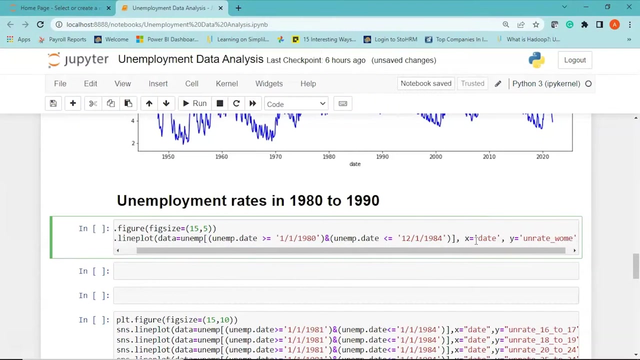 1980 till 1983. now, after that we need to pass in the x-axis and the y-axis. so I'll say x column, for the x-axis to be a date column, and in the y-axis we'll have, let's say, the unemployment rate for women. okay, next, let me run this and we'll see the. 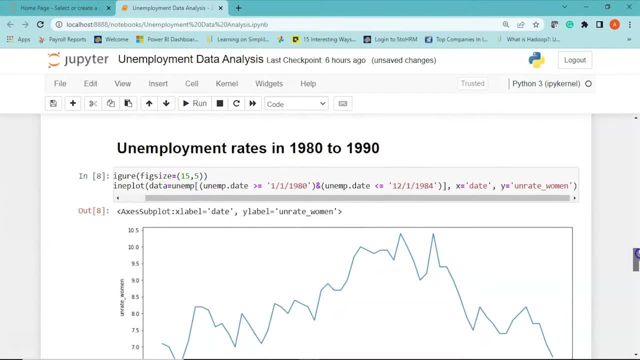 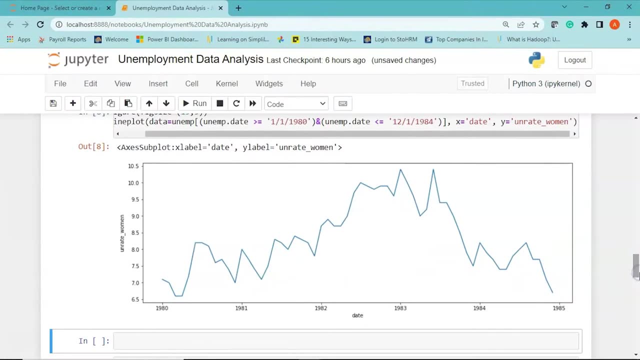 output. there you go. so here you can see the unemployment rate for women between 1980 and 1984. so if you see here, the unemployment rate for women peaked between 1983 and 1984. so now we are going to analyze this data specifically. so let me just give a comment. 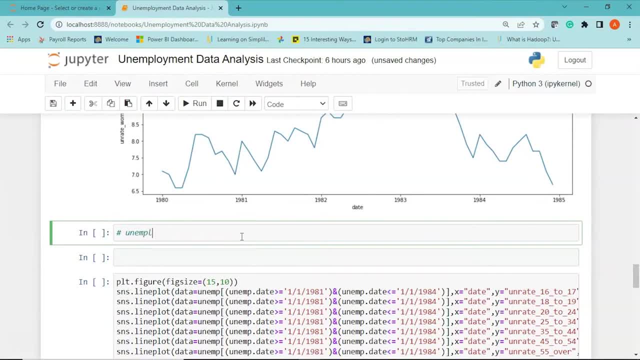 I'll say: unemployment 8 of women between Jan 1982 and December 1983, right? so I'll just copy this above and then we will edit our data. so I'll just copy this above and then we will edit our data. so I'll just copy this above and then we will edit our. 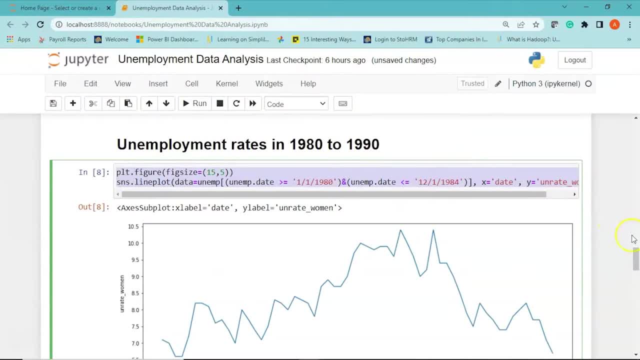 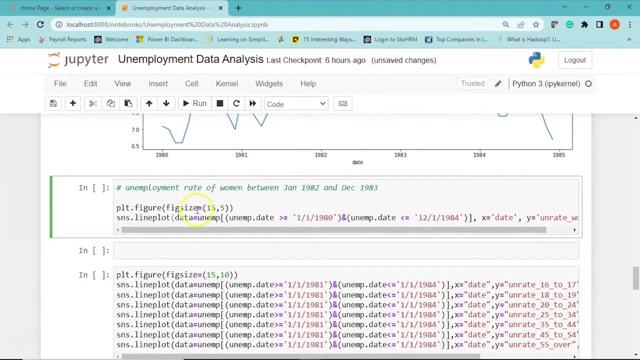 time time it's to cure that the figure size be the same, and then my date should start from 1st of January 1982, because we want to focus on the period that we saw peak, and the next date should be less than equal to 1st of Jan 1984. and the next date should be less than equal to 1st of Jan 1984. and the next date should be less than equal to 1st of Jan 1984. if I you change the date under increasing and reducing, everything remains the same. maybe you can add a. 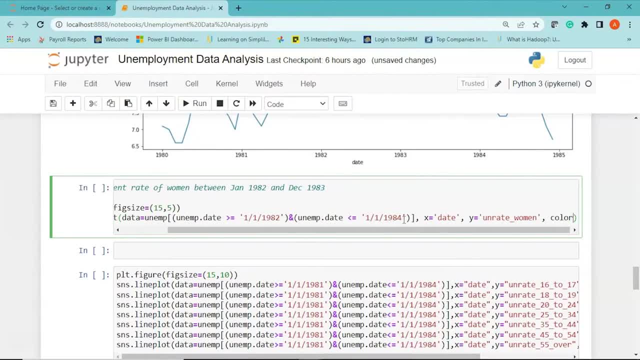 under increasing and decreasing, everything remains the same. maybe you can add a ad color here, so I can add another parameters here and let's see color. we add color here, so I can add another parameters here and let's see color. we want brown if we run it. 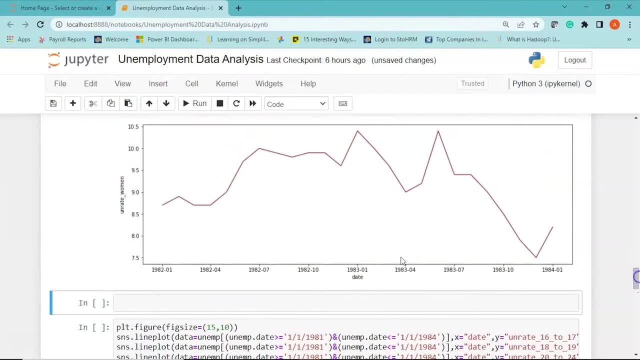 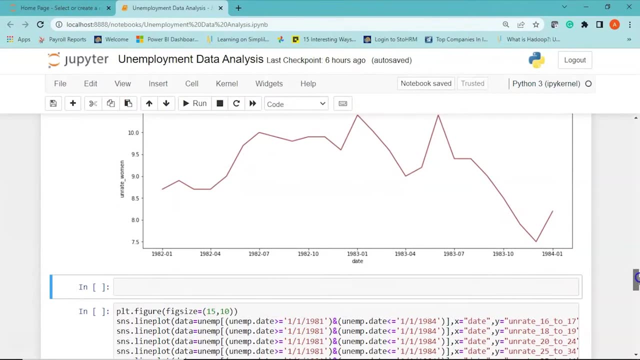 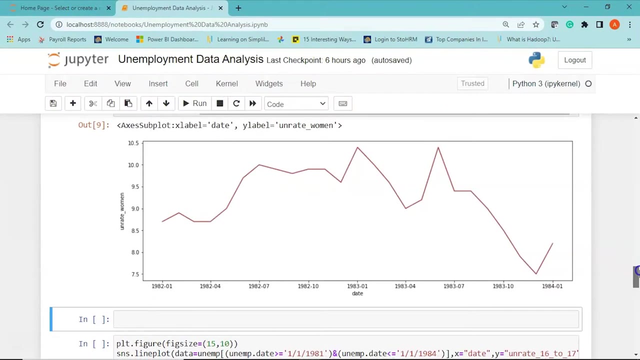 want brown if we run it on on. see the values here. see the values here. És about the unemployed Ε翼 alous in 1983 years blev Quốc bookstore Emily 01 highlight вд 訴. we can check the unemployment rate of men between january 1982 and december 1983. 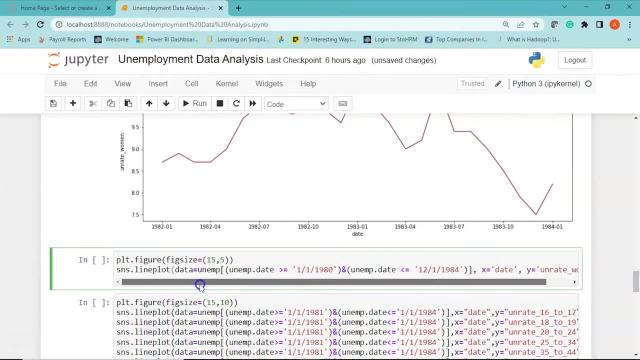 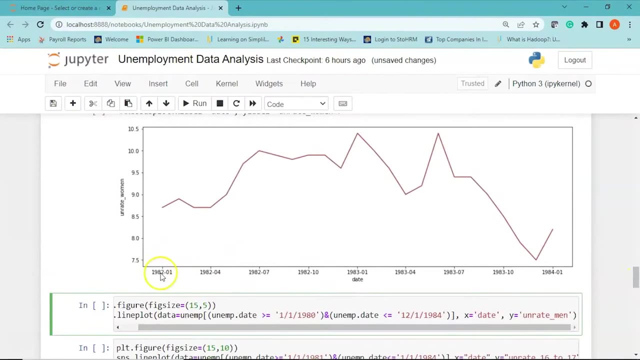 let me just paste whatever i had copied, and here, instead of women, we'll make it men, and the rest remains the same. another thing i wanted to show here is now: if you see this graph, the labels on the x-axis are present horizontally and, if you want, you can rotate the x-axis labels. 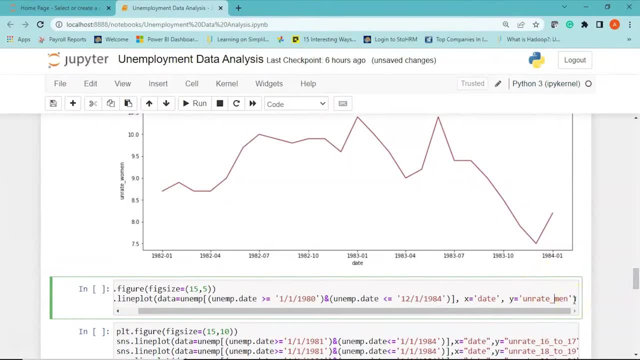 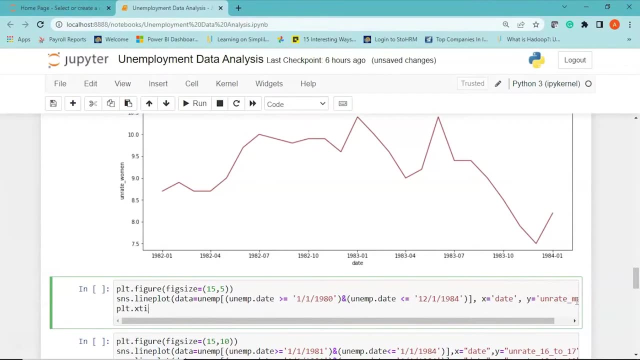 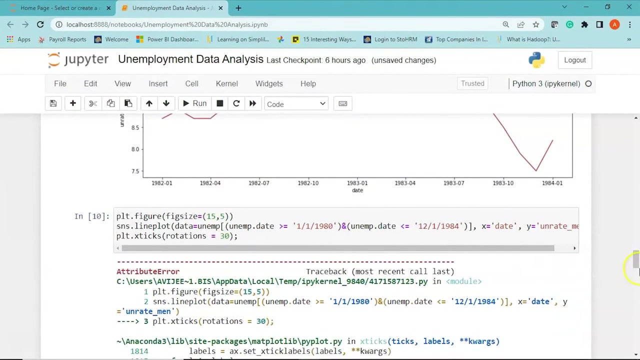 by using the x ticks option or the parameter that we have. so i'll say plt, dot x ticks. then i'll say: rotate it by, let's say, 30 degrees. okay, give a semicolon and we'll run it. okay, it has thrown an error. let's see text: object has no property rotations. 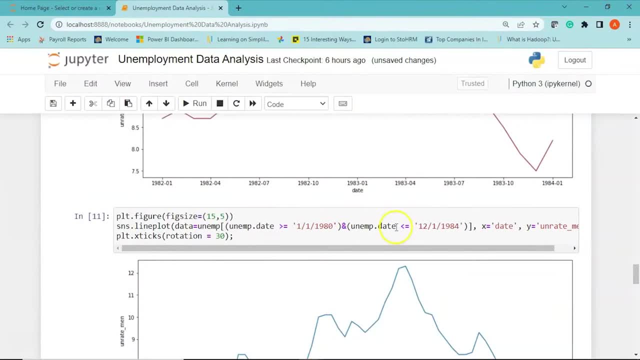 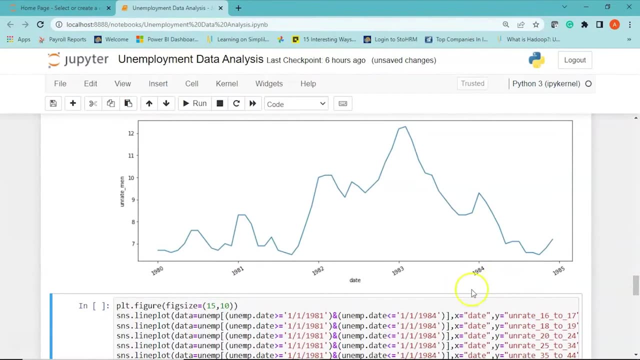 actually this should be rotation. we'll delete the s and run it. there you go. so here you can see. while most men lost their jobs, starting you can say july of 1982, so the unemployment rate increased in 1982 for both men and women. if you compare both. 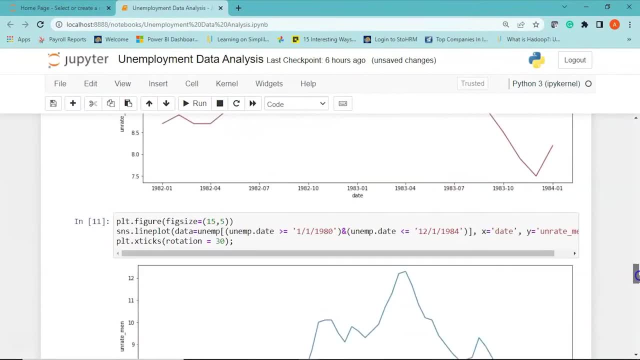 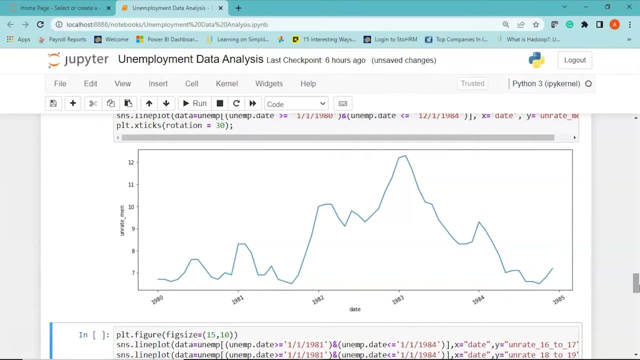 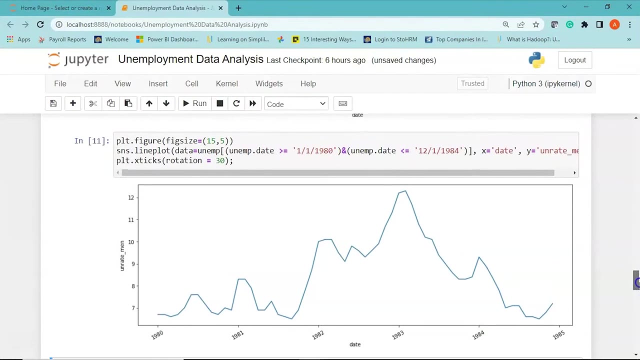 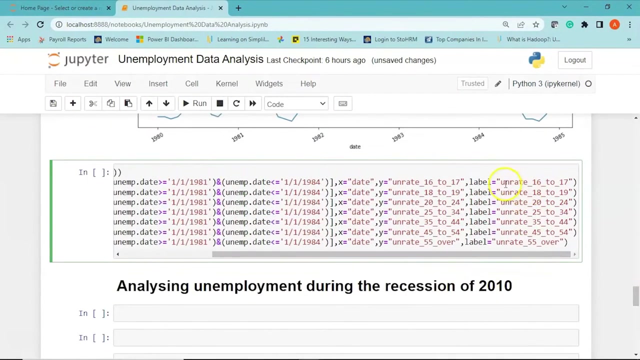 the graphs. so around july 1982 the unemployment rate increased to the highest unemployment rate, which was around 12.5 percent, while women it was around 10.5 percent. now the cell that you see here will segregate the data into different ages. so we saw we have the different. 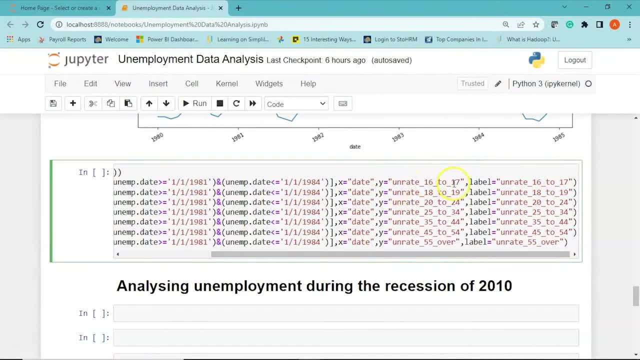 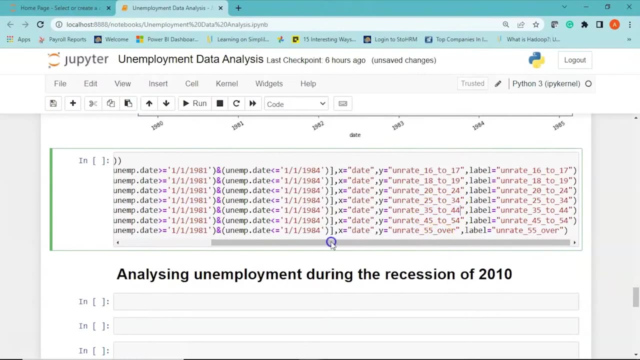 age columns, that is, between 16 to 17 for younger people, then we have the adults between 20 to, let's say, 34, and then you have the data for 35 to 44, as well as 55 and above. so what we are doing here is we are creating line plot for each of the groups of ages and we 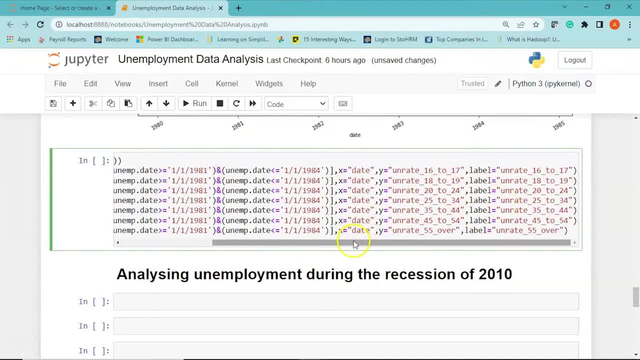 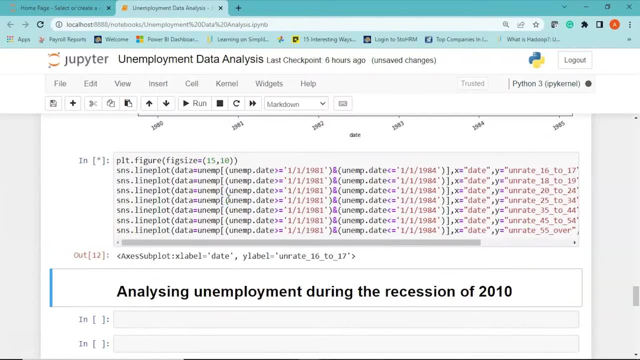 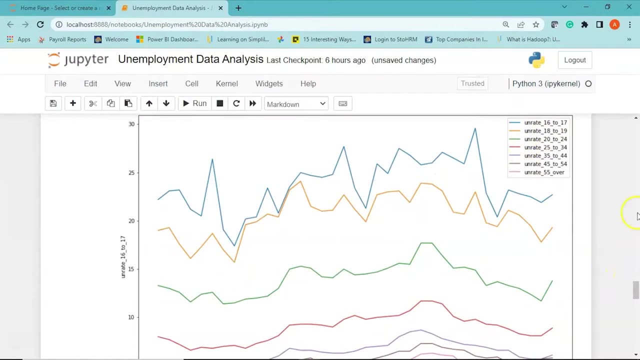 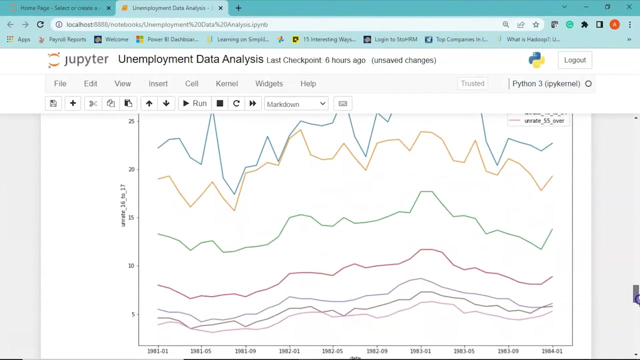 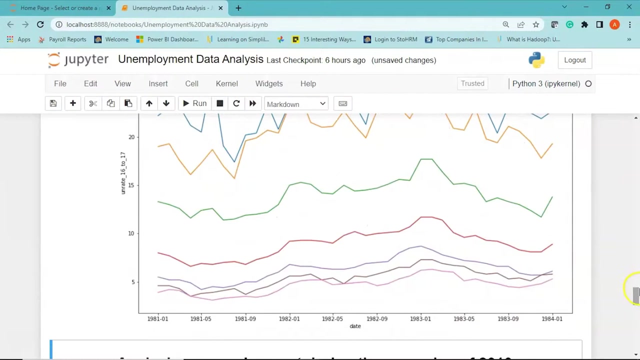 are trying to print them and we have used the labels as well. so let's run this and we'll see the output. if i scroll down, you can see the legend here, the different colors that represent the different age groups. now, overall, if you see the there was some peak after 1983 onwards in. 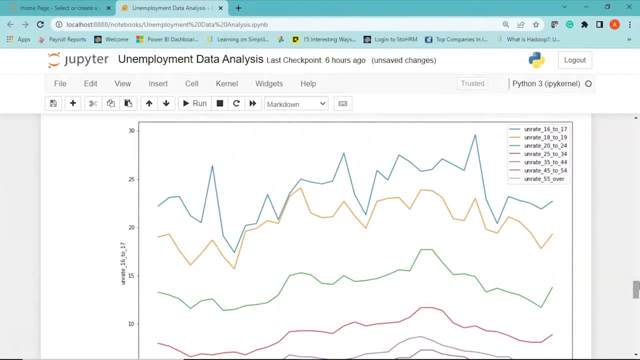 young people. that again points out a fact that more younger people, that is, below 19 years of age, lost their jobs in comparison to people above 20. if you see these blue and the orange line, it represents the younger population between 16 to 19, so they were the most affected during the 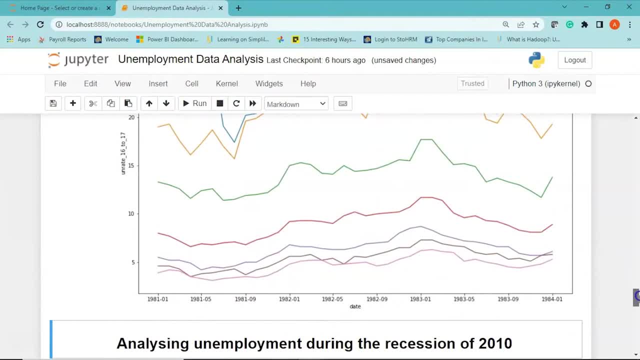 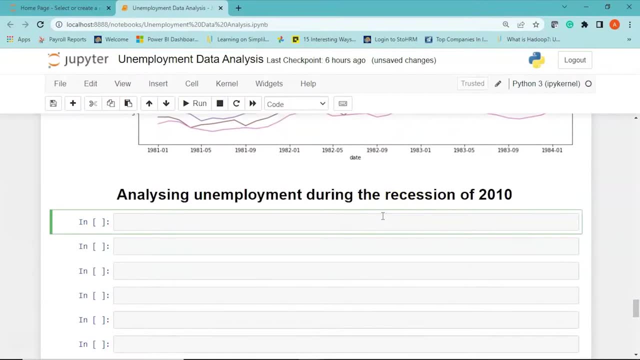 1980 recession. all right, now let's move ahead. and now we are going to analyze the unemployment during the Great Recession of 2010. so I'll create a variable called recession equal to, I'll say unemployment, and, but then square brackets, I'll say unemployment dot date to be greater than equal to. 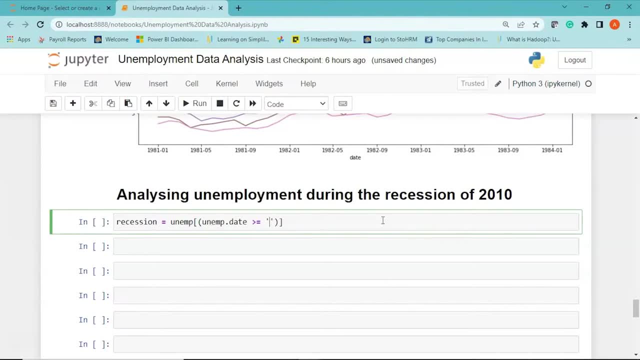 say first of Jan 2009, because that was the time when we had the Great Recession, and then I'll say ampersand, I'll again use another bracket and say unemployment dot date to be less than or equal to, let's say, December 30. 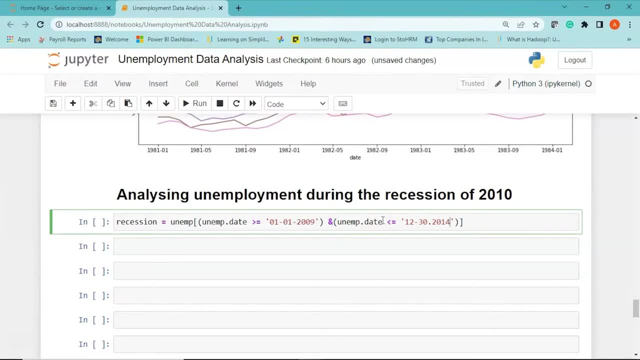 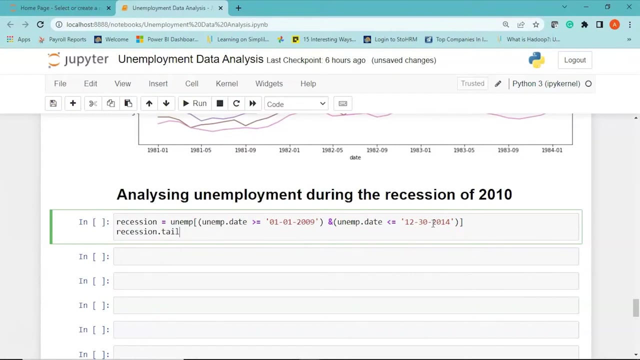 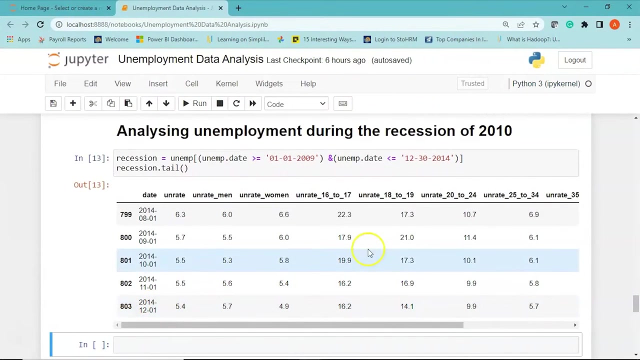 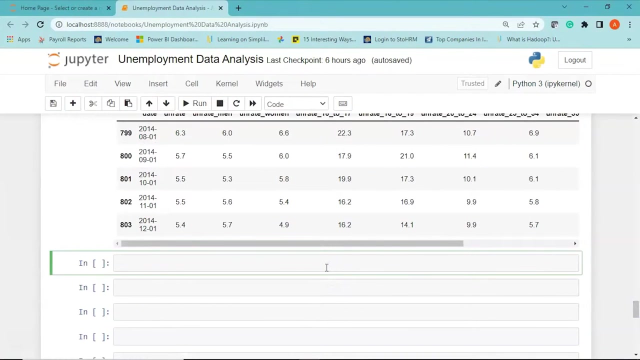 see 2014. cool, this should be a hyphen here. okay, now I'll say recession dot tail. I run it here. you can see the bottom five rows from the data set and we have values till two thousand to fourteen. all right, cool. so now let's visualize the data, that is, the recession data and the overall. 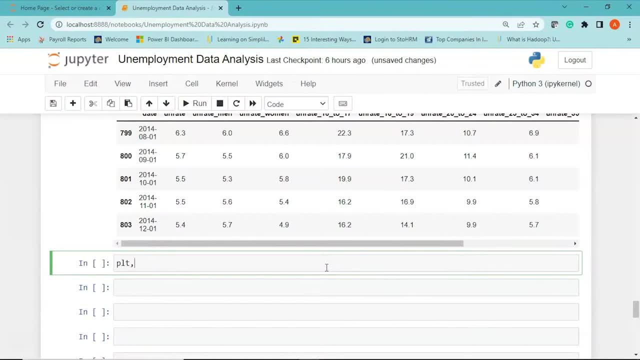 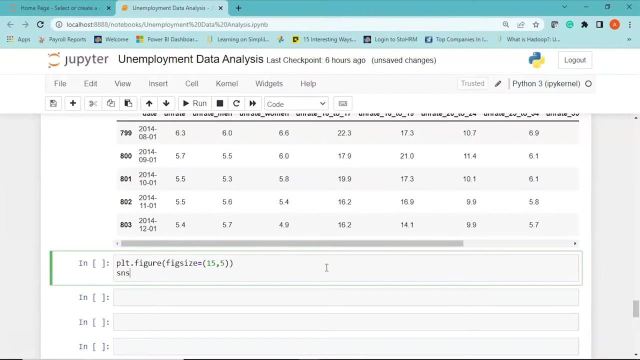 unemployment rate. so I'll say plt, dot figure, and then I'll give my figure size equal to 15 comma 5. next I'll say sns, dot line plot, and I'll say my data to be equal to recession comma, my X to be date and my Y to be. 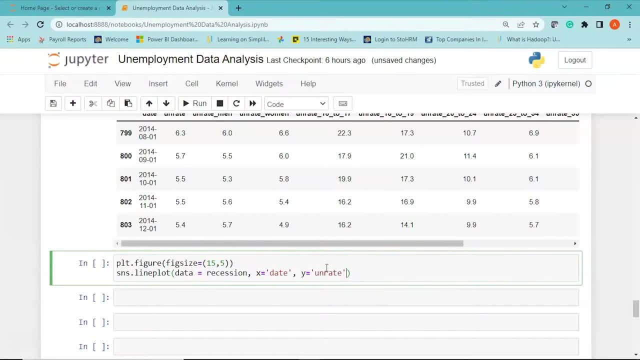 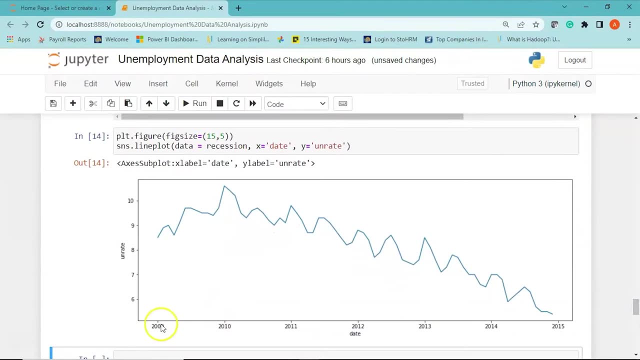 rate column. now let's run it and you can see the result here. so between 2009 to 2015, you can see the date below r. what is ев? the result here- so between 2009 to 2015, you can see- was a clear spike, and the unemployment rate in the united states went close to 11 around 2010. 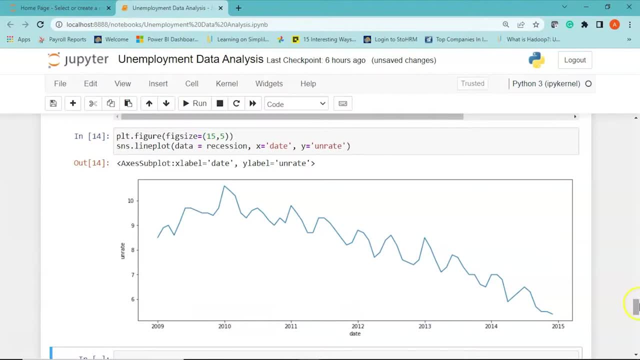 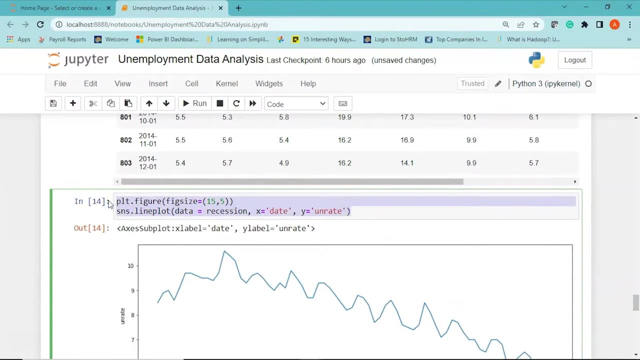 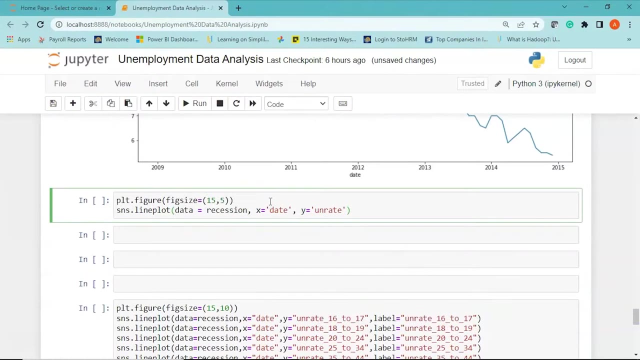 that is, mid of 2009 and 2010. now we are going to visualize the data individually for men and women, as well as for the different age groups, so i'll just paste my above cell here and now. let's change the y axis to unread underscore men. 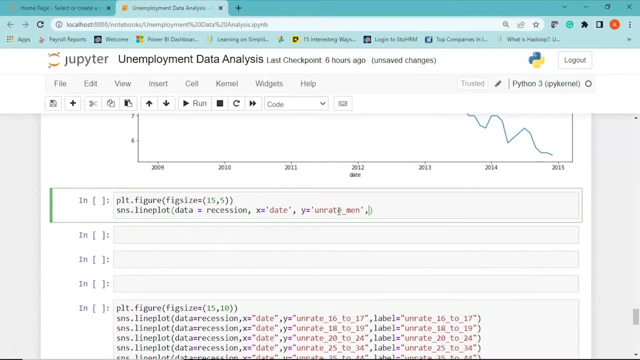 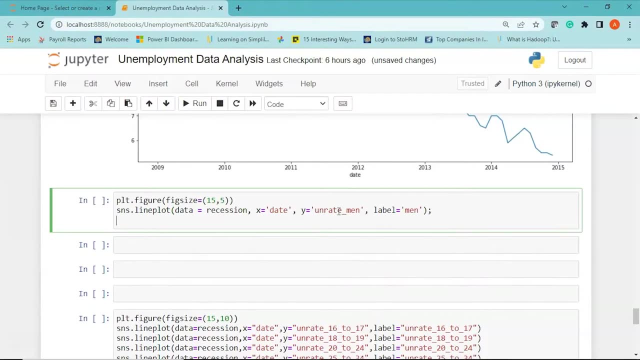 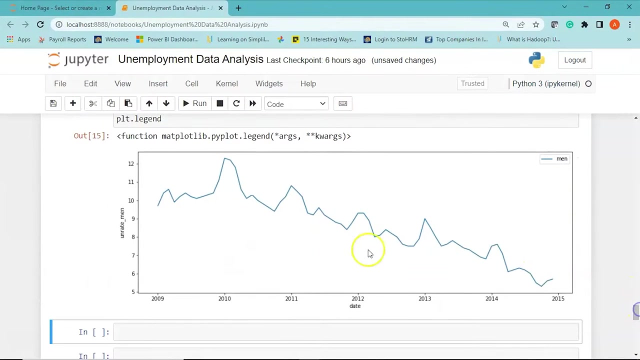 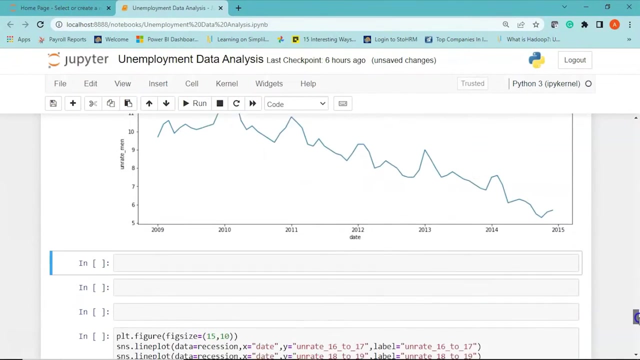 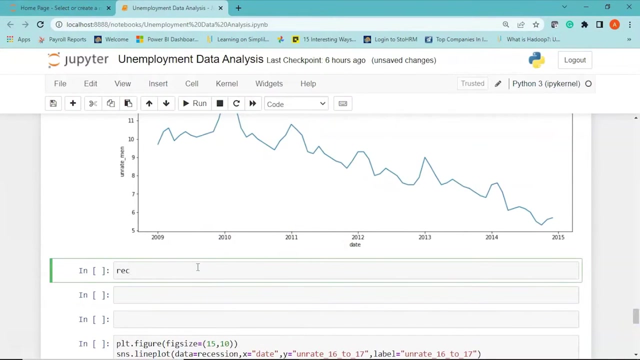 i'll say let's say add a label called men, let's also give the legend so that men displays on the top right. so if i run it here you can see we We have the unemployment graph for men who, if you see the statistics for recession on, 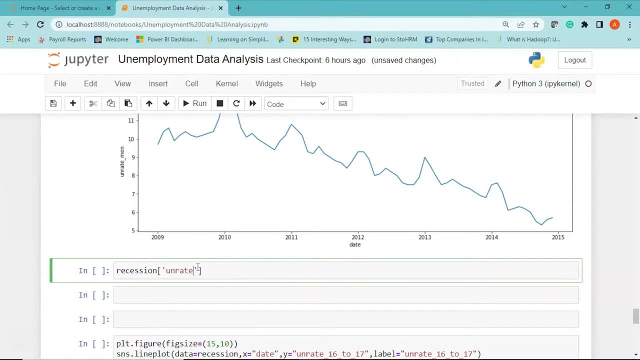 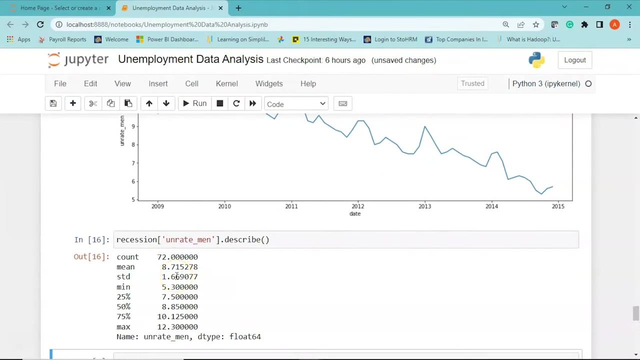 the unemployment or the unemployed men during this specific period. Use, describe, function and run it. So here you can see the values. So the average unemployment rate was around 8.7% during this period. The maximum was 12.3%. If you see the graph, this is around. 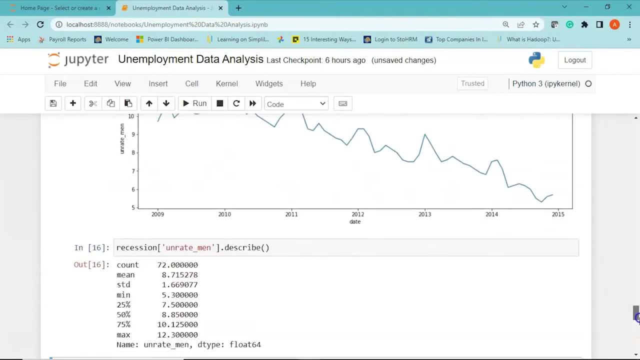 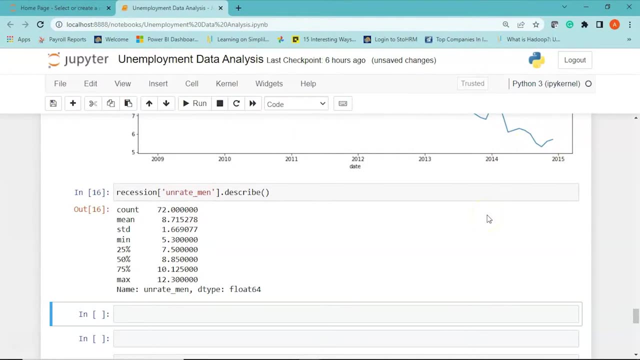 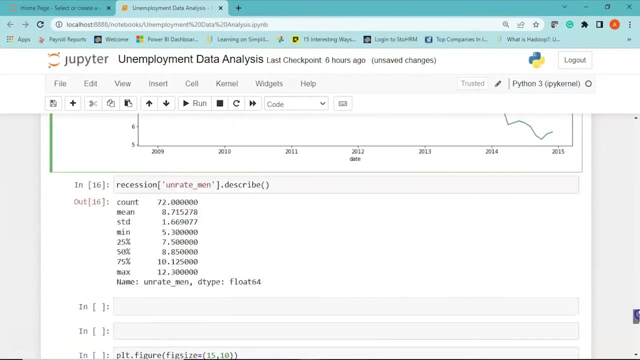 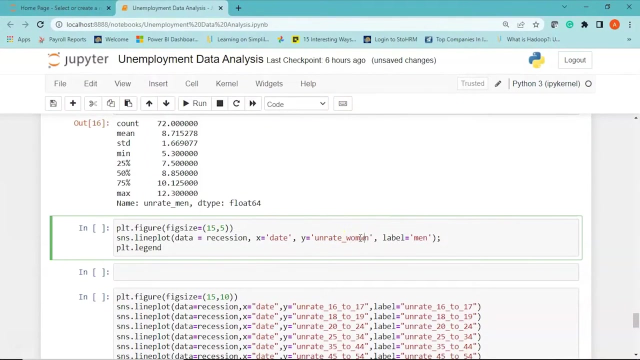 12.3%. This is the peak, and the minimum unemployment rate was 5.3%, which is this part All right. And similarly, we'll now check for women, So I'll just copy this and paste it here. We'll edit the y-axis, I'll say women and I'll edit the label as women. 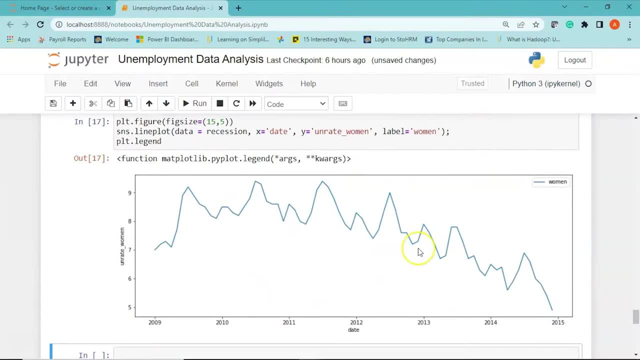 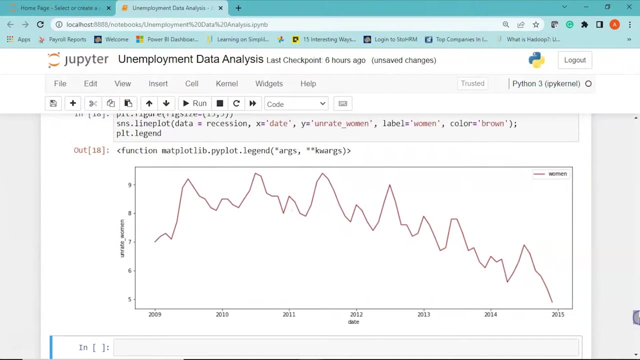 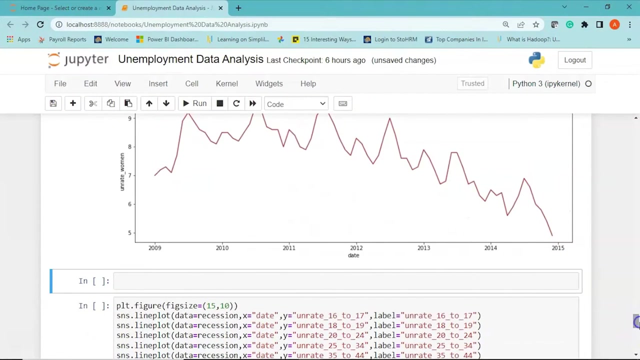 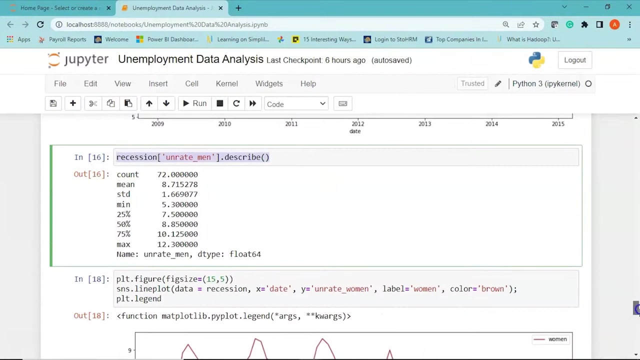 Let's run it and you can see the output. here Want you can add a color, Let's say brown. You can now see the unemployment rate of women during this period between 2009 till 2015.. Now again, let's use the describe function over the column unemployed rate of women. 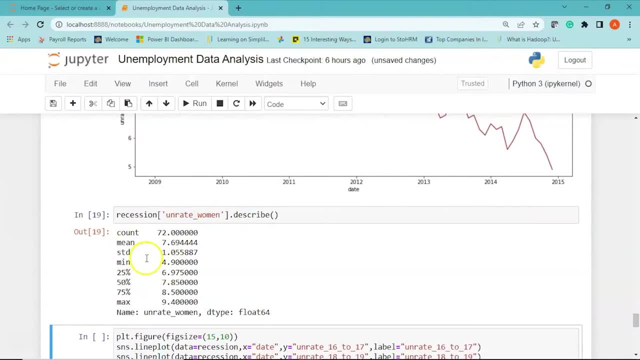 So I'll just edit this to be women. You can see here: the average unemployment rate for women during this period, that is, of the greater section, was 7.69%. The maximum was 9.4% and the minimum was 4.9%, or close to 5%, which is this value. 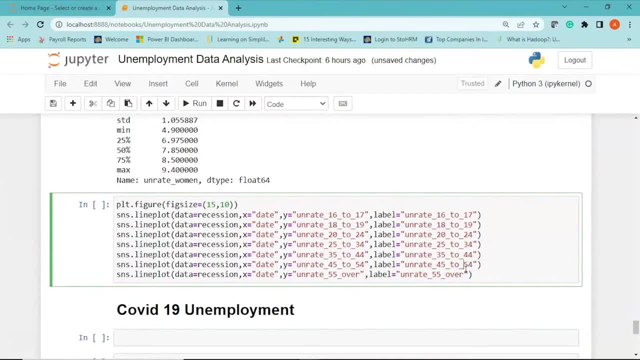 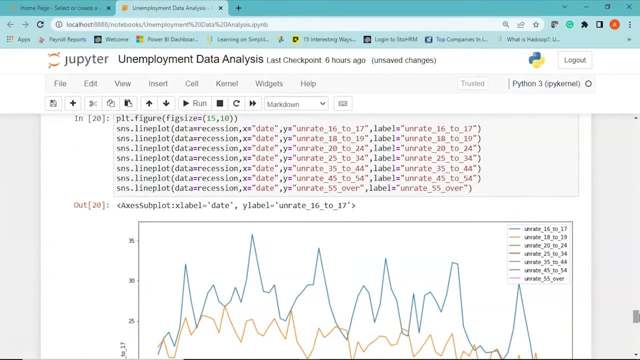 Cool. The next cell. as we did above, we are now categorizing the unemployment rate based on each group. So starting from 16 till 55 and above, Let's run it and you can see the output here. So the unemployment rate touches around 35%. 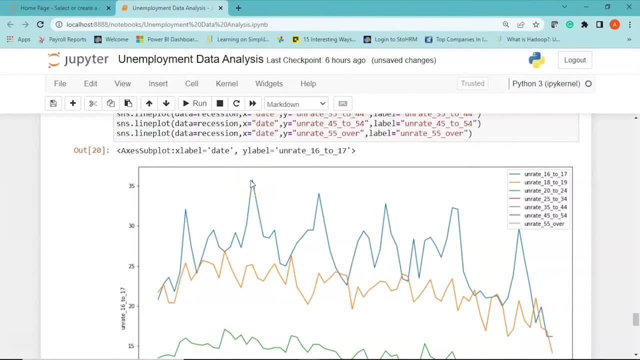 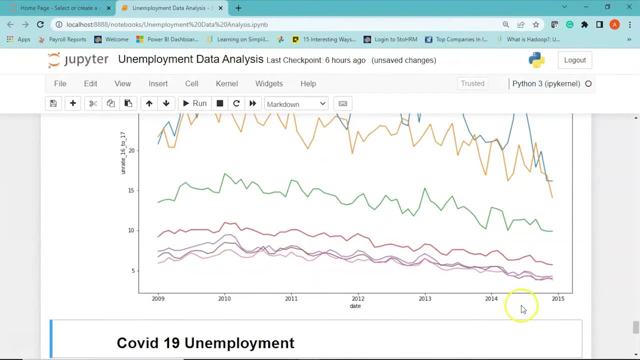 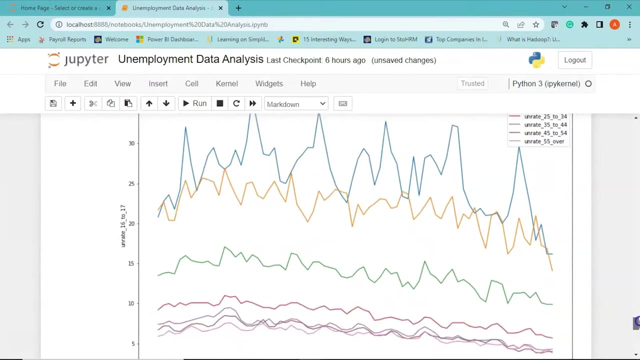 You see here it was around 35%. So the unemployment levels touched at least sky high during 2010.. If you see this, this is around 2010,. it was around 35% for the eligible youth. Those were unemployed And after that you can see the unemployment rate. 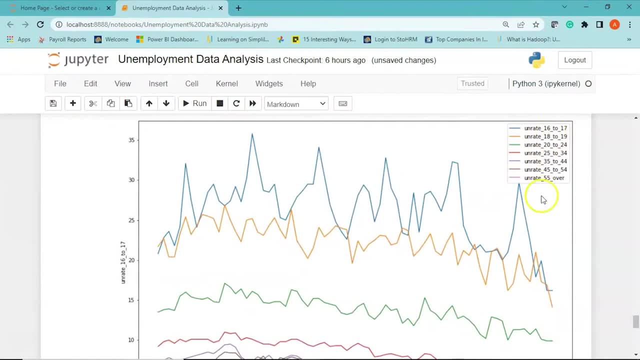 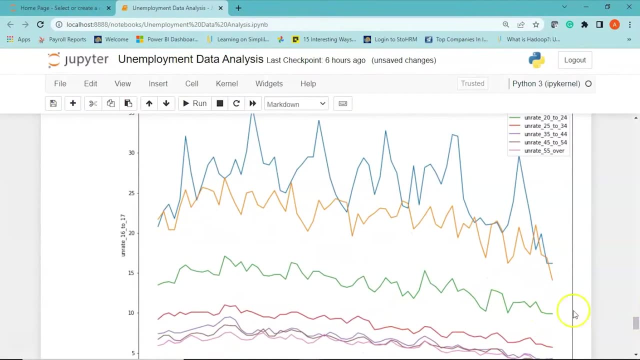 Let's see the unemployment rate, that you have the second age group, which is between 18 to 19, who are the most affected, followed by 20 to 24, and then you have 25 to 34, and so on and so forth. great coming to our 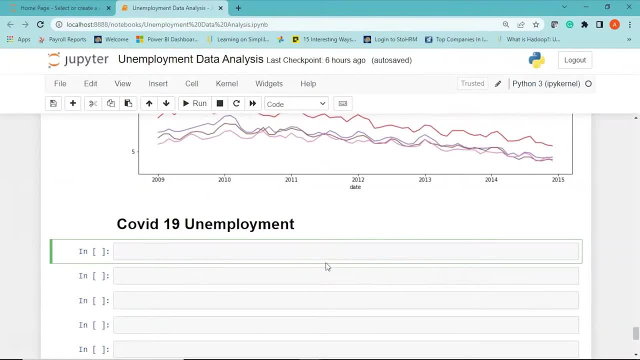 final section, where we'll analyze the data around the covid 19. so this is the beginning of 2020, when the world was hit by covid 19, so i'm going to filter the data, so i'll create a variable called covid underscore 19, i'll use my original data frame, which is unemployment, and then 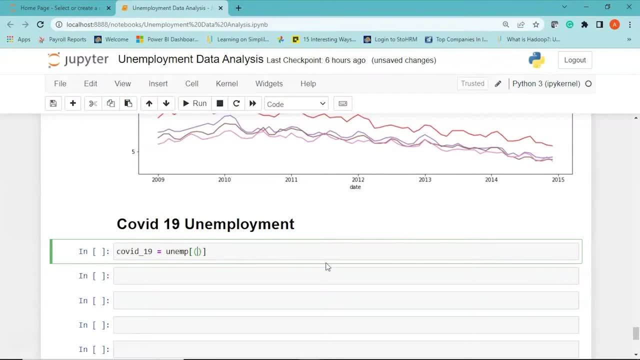 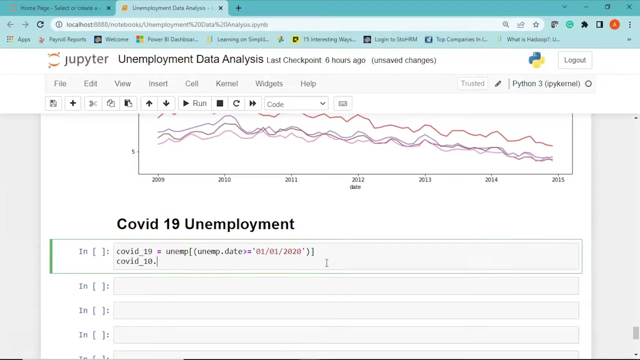 i'll give square brackets and within braces i'll say unemployment dot date to be greater than equal to. it should be greater than equal to, let's say first of jan 2020. okay, now let's print my covid 19 data set. i'll say covid 19 dot head. so here you can see. our data starts from first of 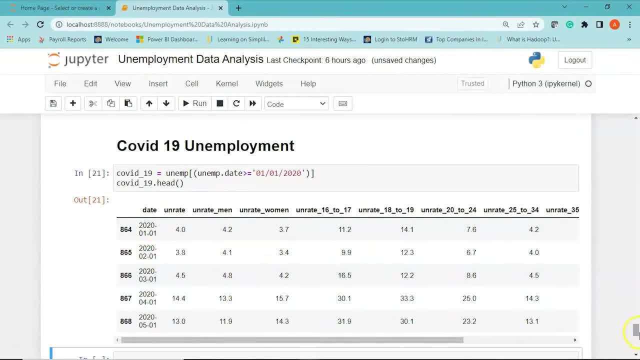 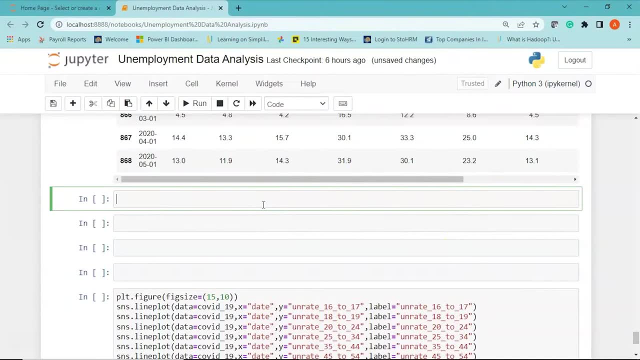 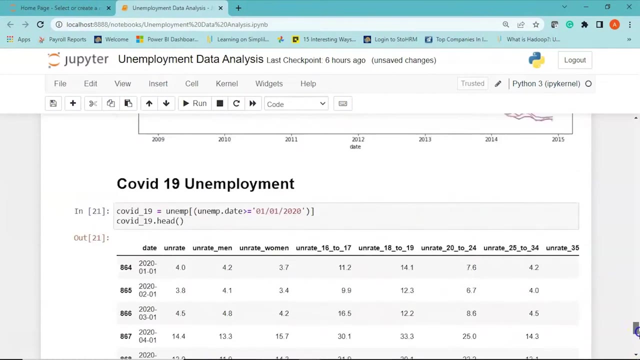 jan 2020, then second of jan 2020, third, so on and so forth. great, now here let's first analyze the data for unemployment rate for men. i'll just copy one of the cells above and i'll paste it, and then we can edit it. let's say i'll copy this: 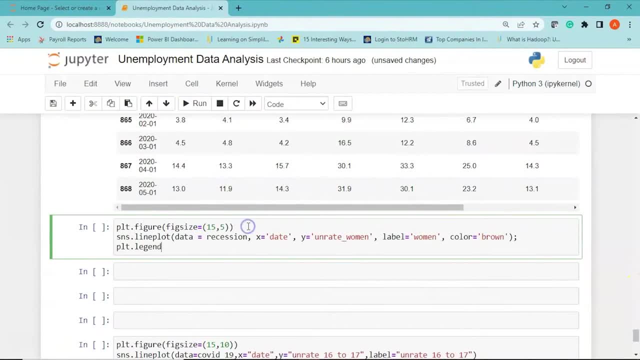 and then let me just paste it here. so let the figure size be 15.5 and data: instead of recession, we are going to use covid 19.. okay, next, my x column will be the same, that is date, and my y column will have unemployment rate of men. label would be men and let's say i'll have a color of. 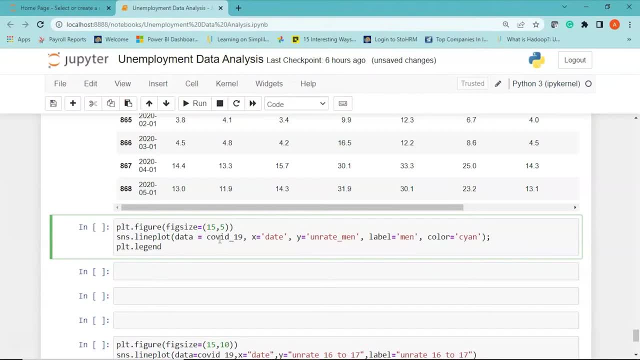 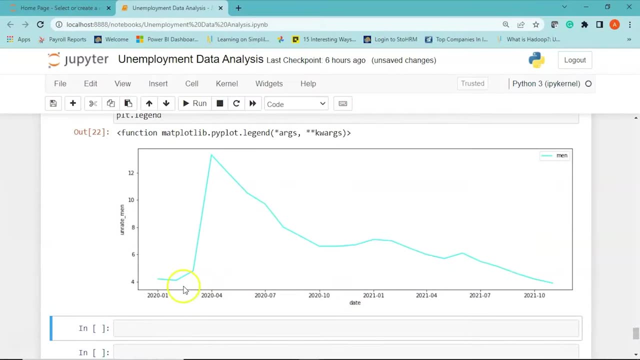 let's say: i'll use cyan and we'll give pltlegend, let's run it. there you go. so if you see this graph clearly, around march and april 2020, there was a huge spike in the unemployment rates in the united states for men, which crossed nearly 13 percent, and around july- late july and october- between 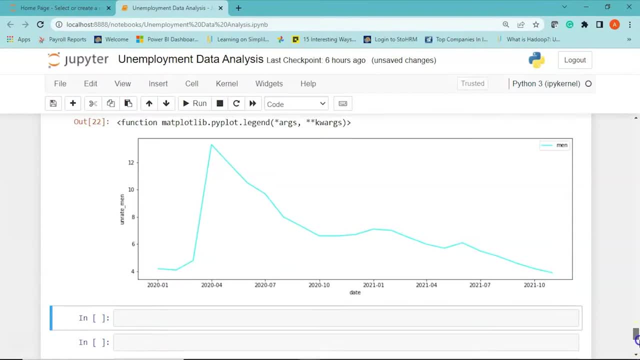 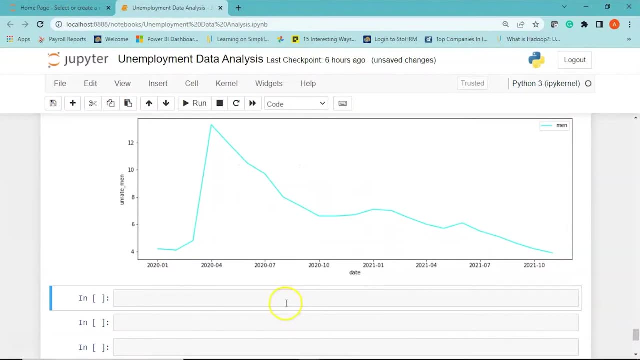 late july and october it started decreasing. so this was the time when us was hit by the corona virus wave. great, i'm going to use the describe function again over the unemployment rate of men. so i'll say covid underscore 19, then i'll say unrate underscore men dot. 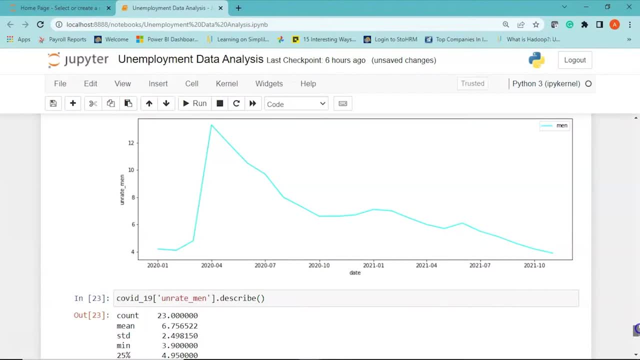 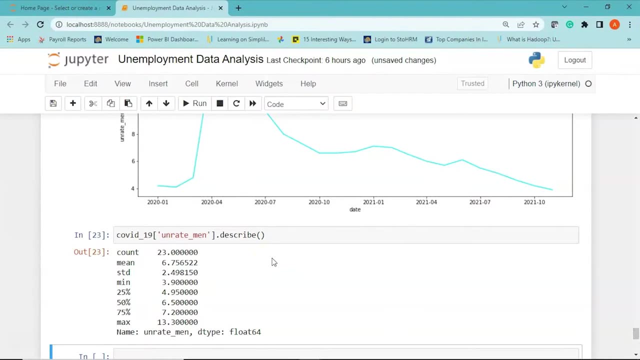 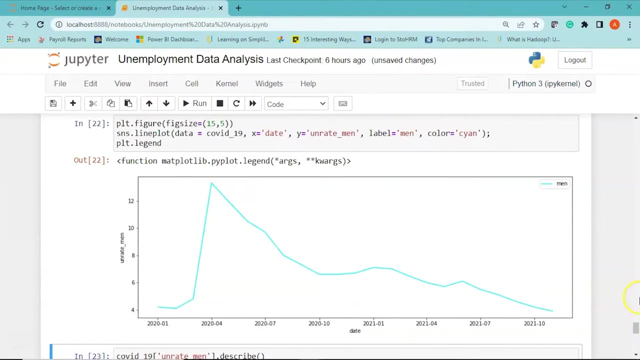 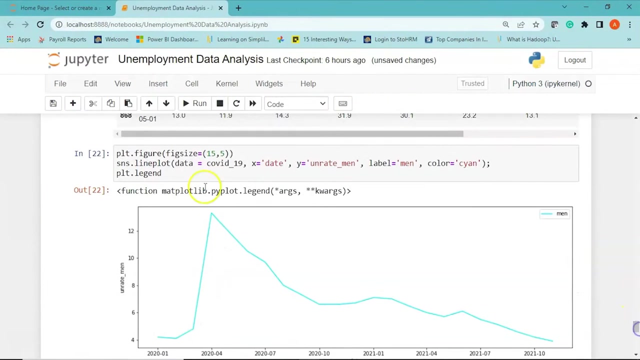 describe. if i run this and scroll down, you can see here: most men lost their jobs in march 2020, with unemployment rates peaking at around 13.3 percent. that you see in the graph here, which is the peak point, is around 13.3 percent. okay, similarly, let's do it for women as well, so i'll 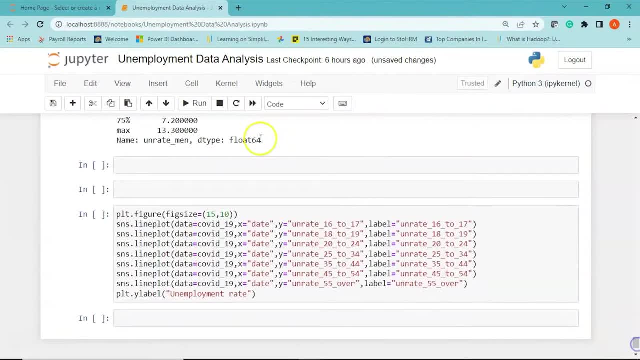 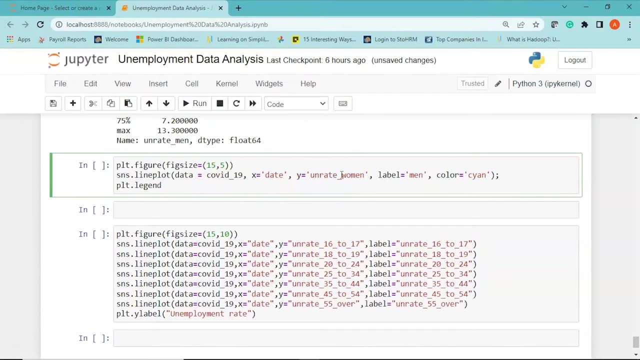 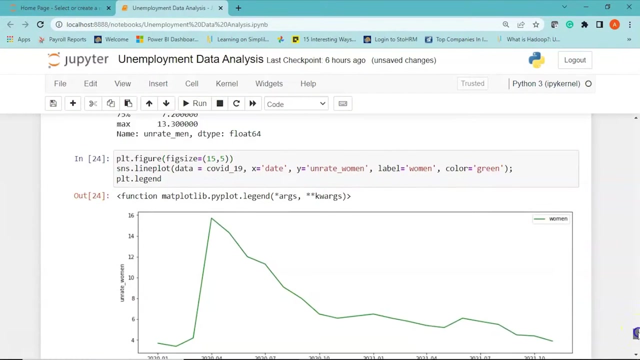 just copy this code and paste it here now: instead of unemployment rate for men, we'll say unemployment rate for women, and label would be women. we can use a color, let's say green. okay, let the legend be there and we'll run it now. if you look at this graph closely, what you see is there was a huge spike again during. 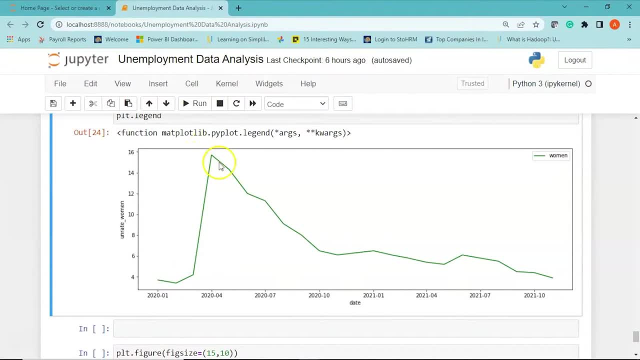 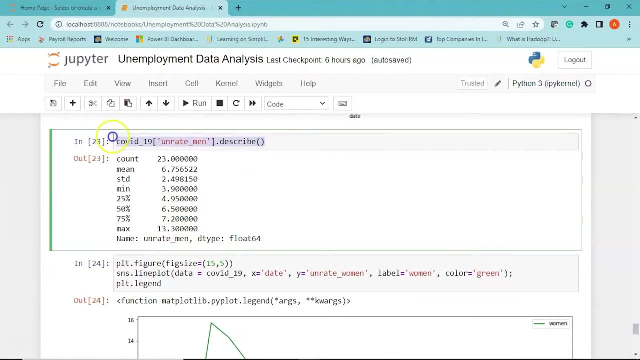 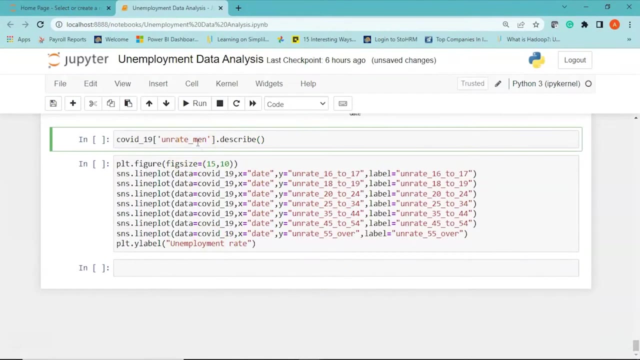 march and april 2020, when the cases started rising in the united states, and for women it was around 15 percent compared to men, which had 13.3 percent. now, if i use the describe function and replace this with unemployment rate for women and run it, 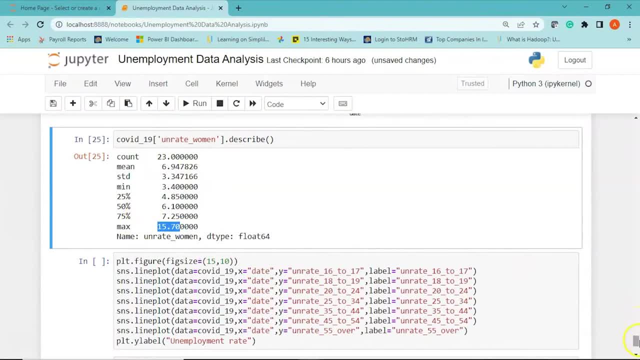 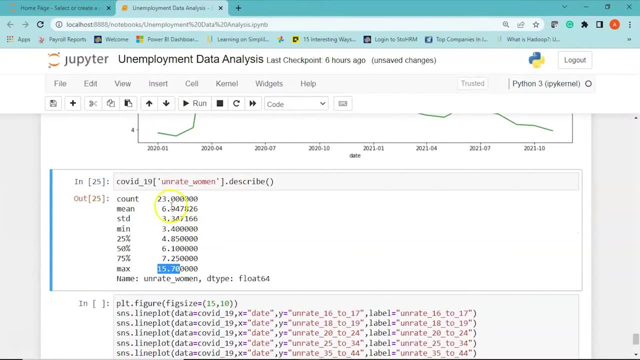 you see here, the maximum value it's touched was close to 16, which is 15.7. so this value is 15.7 and the average percent was 6.9. that is, close to 7 percent of unemployment throughout this period. all right, now let's see the unemployment rate for women. 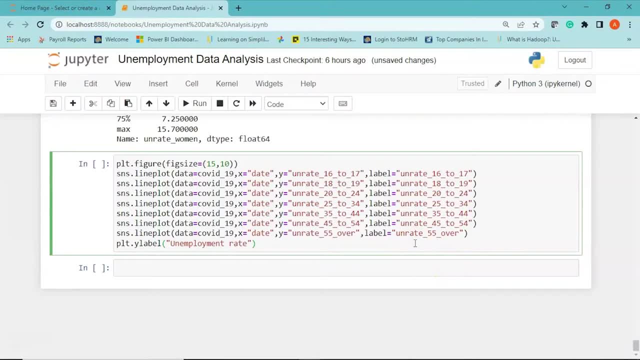 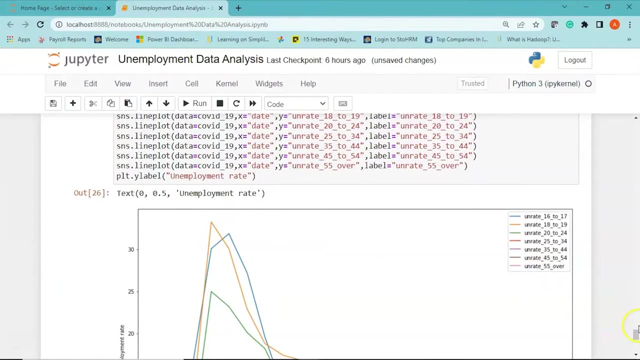 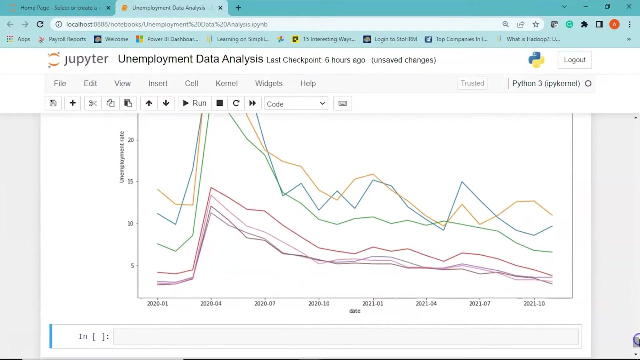 the final cell. we are again segregating our data into different age groups and we'll see what age group was impacted the most during the coronavirus pandemic. let's run it okay now. if i scroll down, you see here the orange line represents the unemployment rate between 18 to 19 years of age. so during the coronavirus pandemic, that is, around march and april 2020. 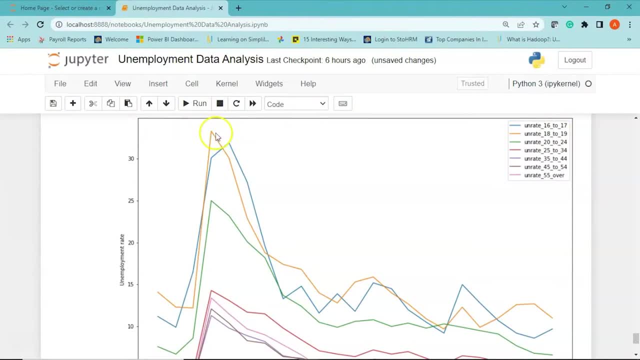 this age group, between 19 to 18 to 19 years of age, were the most affected, that is, around 33. after that we have the age group between 16 to 17, which is again over 30, followed by 20 to 24, and then we heard the other gauge groups as well. so most women lost. 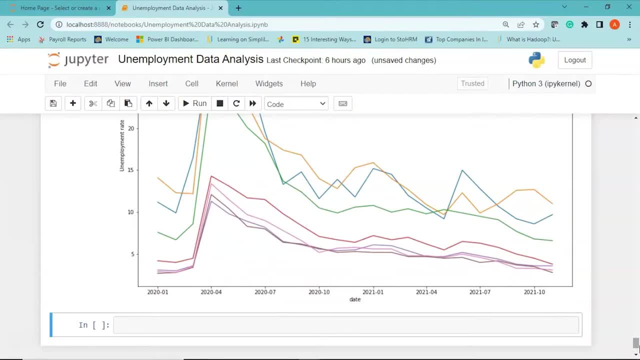 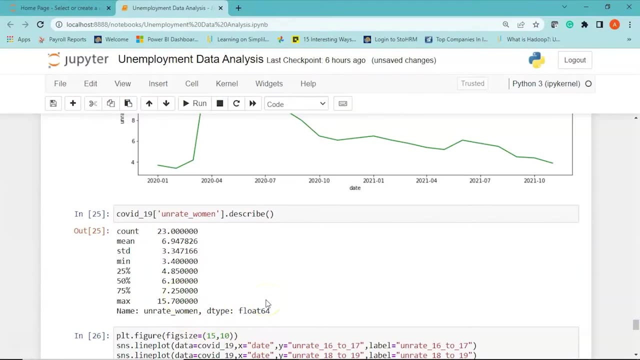 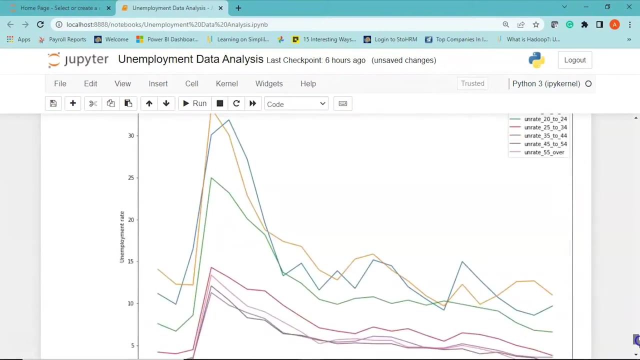 their jobs in march of 2020, with unemployment rates peaking 15.7 percent. that we saw just above 15.7 percent. so from the above data, it is evident that women were most affected by the pandemic. so i hope this demo was useful for you in creating an analysis, an exploratory. 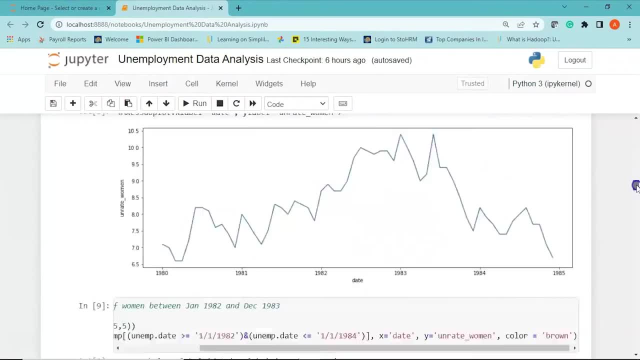 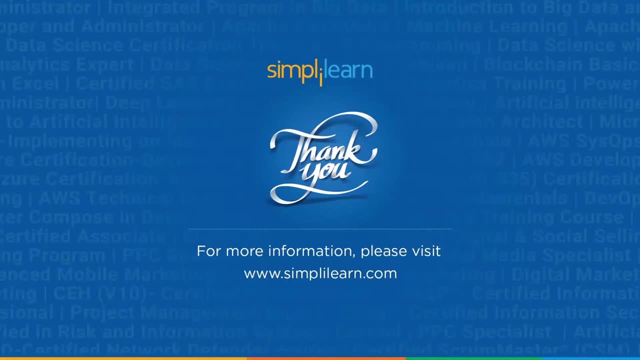 analysis using a time series data. we saw all our graphs based on date and time, and that brings us to the end of our demo session. hope this video was useful and informative. if you have any queries, please feel free to put them in the comment section of the video. thank you for. 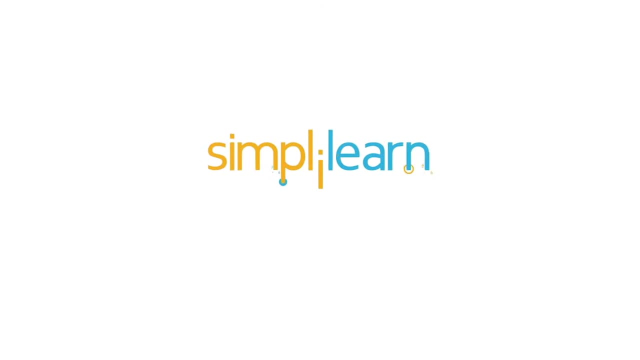 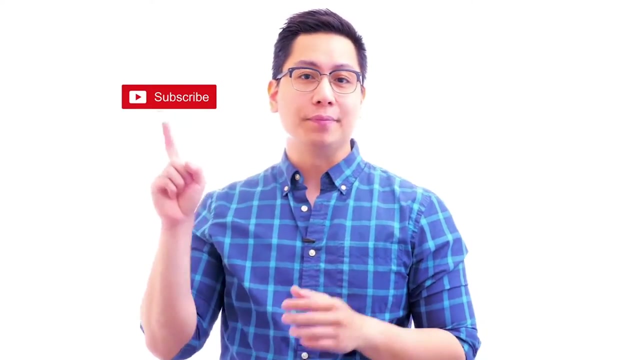 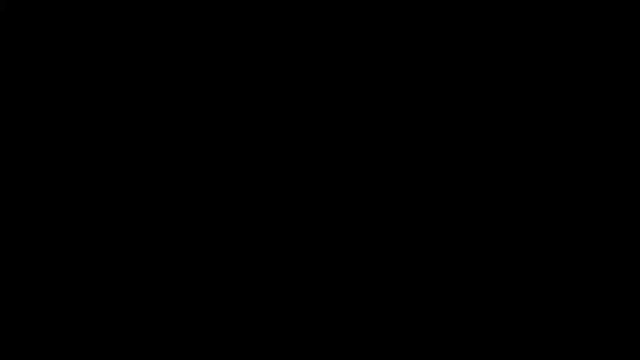 watching, stay safe and keep learning hi there. if you like this video, subscribe to the simply learn youtube channel and click here to watch similar videos, to nerd up and get certified. click here to watch more videos like this one, and don't forget to hit that like button and hit the bell icon. 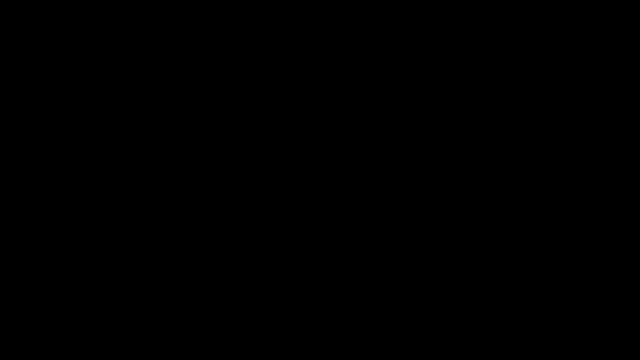 so you don't miss any of the future videos and i'll see you in the next one. bye you, you. 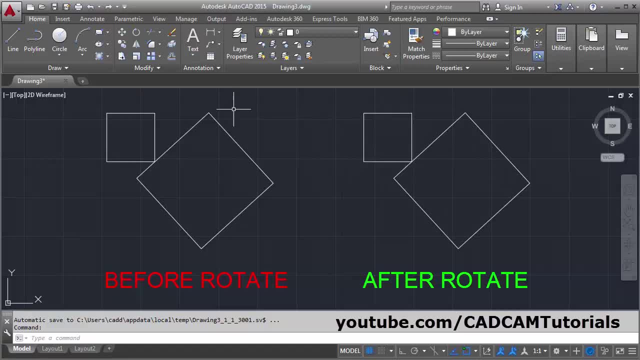 I want to rotate this object. To align these two lines, click on rotate, Select the object, Enter, Give the base point around which you want to rotate. Then click on reference, Then give the reference angle. I want to align this line. Therefore, click on two points of this line. This is first point. This is second point. 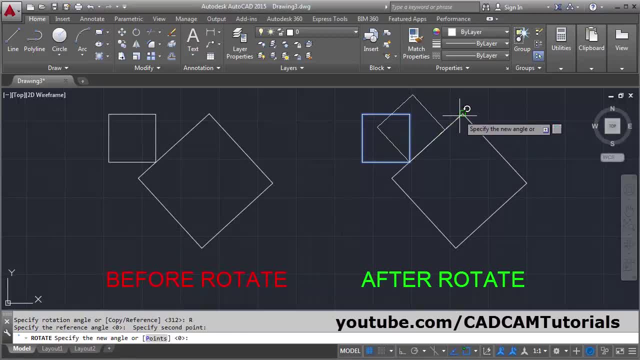 Then give the new reference I want to align with this line. Click on the end point of this line, So the object will be aligned with this line. That's all. Thanks for watching. We will stop here.